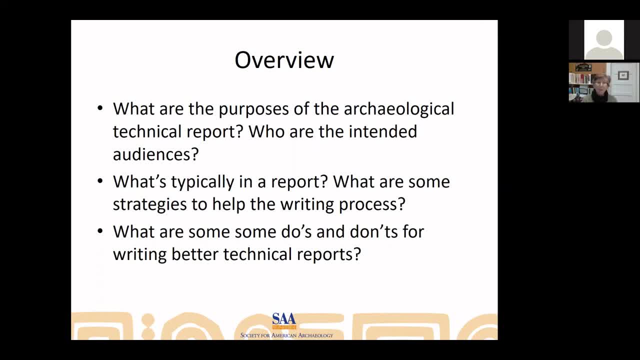 you need a plan for the archaeological investigations. you need a plan for summarizing the results. So today I thought we could break down this big project into doable pieces. We'll look at some strategies and resources that'll help you organize and write that technical report, especially for cultural resource management. 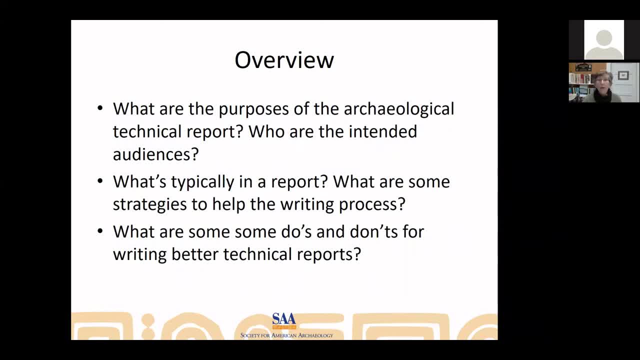 So first we're going to look at why you're writing it and for whom. Next, we're going to look at a typical report outline And finally, I'll give you some do's and don'ts, mainly from my perspective as someone who may be reading your report. 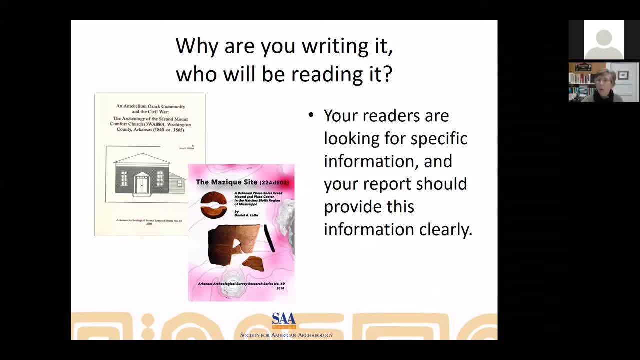 All right, Well, first, what are the purposes of this report And who's going to be reading it? Typically, you're writing to satisfy the requirements of a contract or a grant. The client or the sponsor expects a report after funding the work. 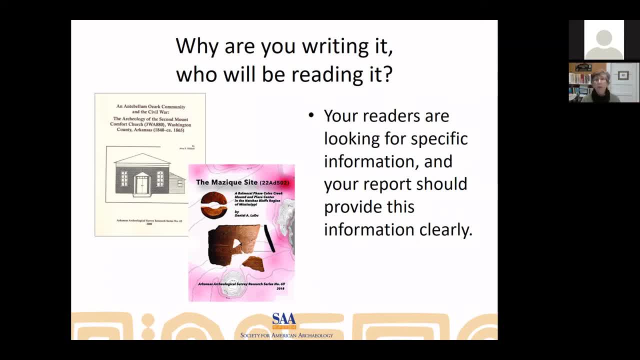 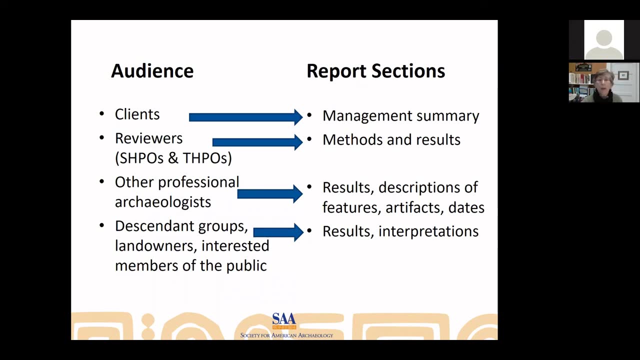 So you're telling what you did, what you accomplished, why it's important. Now there's several audiences that you want to consider First. clients need to make decisions about whether they have to do further archaeological work or avoid significant sites. They're going to be looking at the management summary for key points. 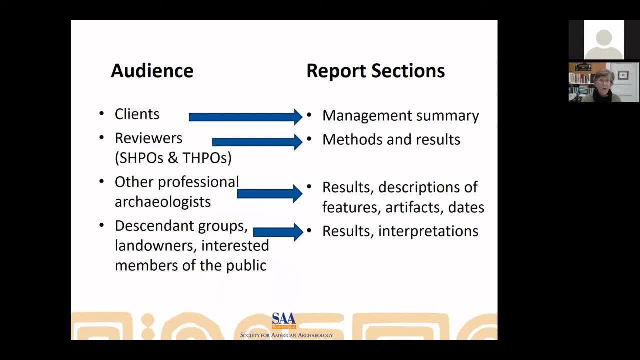 Reviewers. those would be the State Historic Preservation Officers, Tribal Historic Preservation Officers. These people are going to be making decisions. They're making recommendations about site significance and National Register of Historic Places eligibility. So these folks are going to be looking at the methods that you're using and the results that you got. 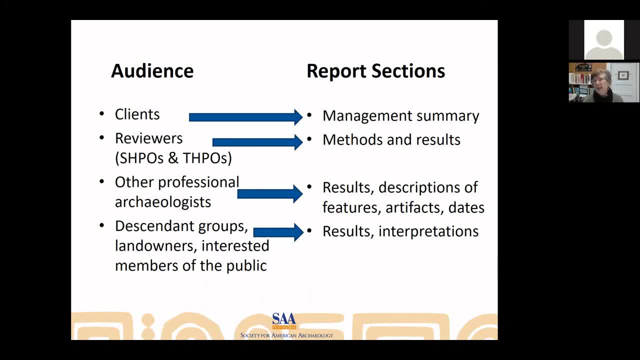 Other professionals like me. we're going to be interested in the descriptions of what you found so that we can make comparisons with our own work in this region. But there are other readers too that you should consider. There are members of descendant groups who are interested in the interpretations that you've made about their history. 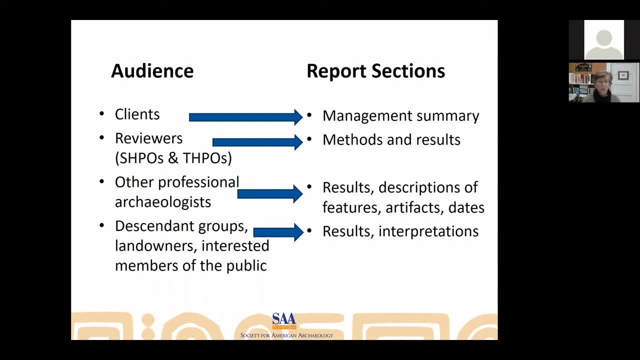 There are landowners who are interested to learn about. does anyone care about the mound in their field And why should they preserve it? Recognize that only some of your readers will be professional archaeologists. If you think about your audiences, you need to be clear, you need to be straightforward, you need to explain terms when necessary. 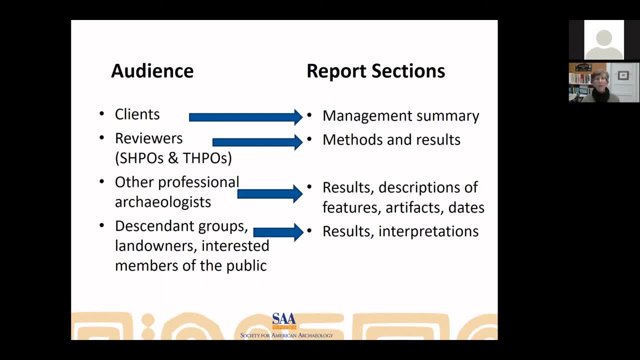 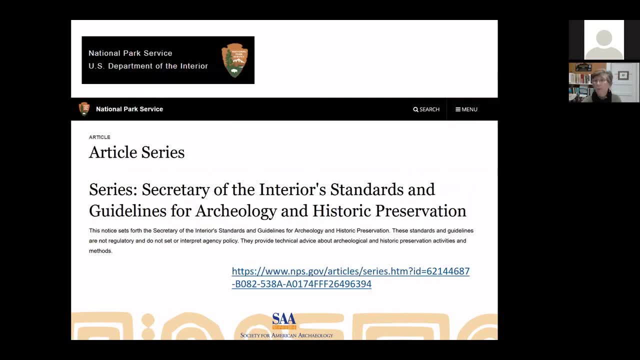 But assume that people are knowledgeable and interested in what you have to write. So in 1983, the National Park Service developed and published the Secretary of the Interior's Standards and Guidelines for Archaeology and Historic Preservation. This included an outline for technical reports in archaeology. 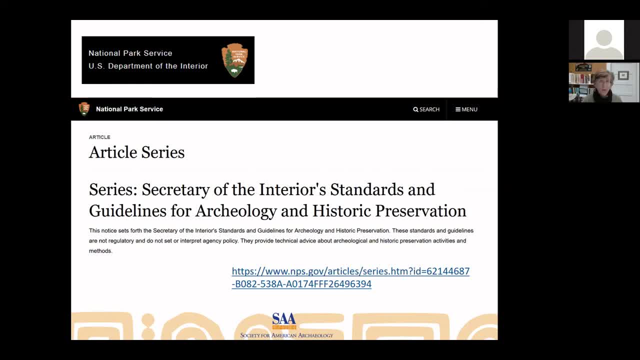 Since then, states and even some counties have published standards and guidelines for field work, for reporting and for curation as well. These typically include sample report outlines with sections for background methods, results and recommendations. Why are these important? Again, your readers will be looking for specific kinds of information. 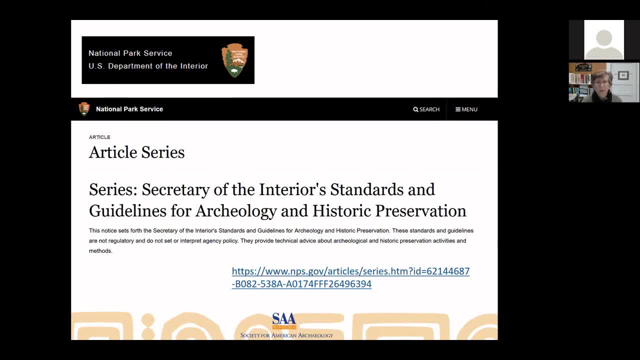 They're expecting specific kinds of information on which to base their decisions. Were there enough shovel tests dug to find subsurface indications of archaeology? What artifacts did you find that showed the site was 6,000 years old? What factors did you use to base your determination of eligibility? 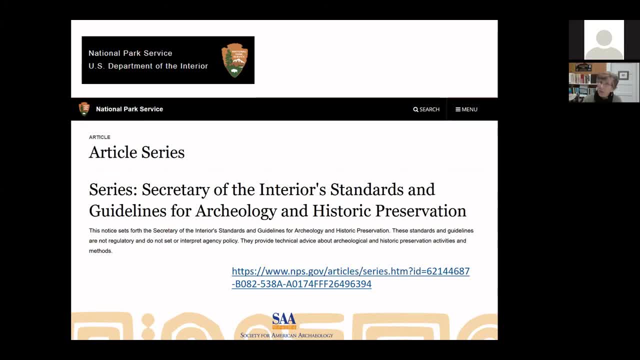 Are we going to have to move the right-of-way to avoid significant sites? So your readers are going to be expecting certain kinds of information. You want to have answers to their questions in your report. Do you want to have a map of the sites? 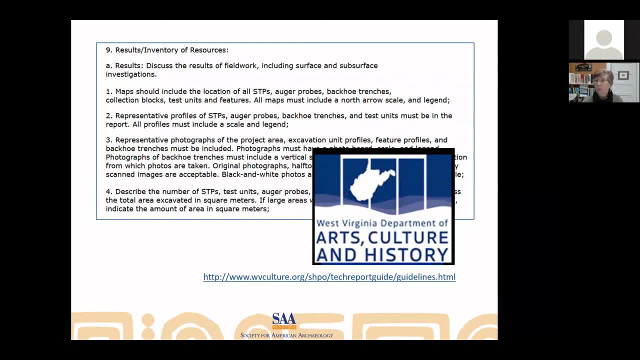 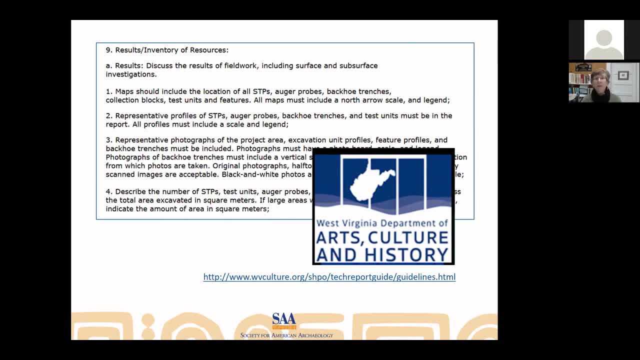 So take a look at the ones for the states that you're working in. As you can see from this excerpt from the West Virginia Department of Arts, Culture and History, the guidelines can be quite detailed in terms of how the SHPO expects field work to be done. 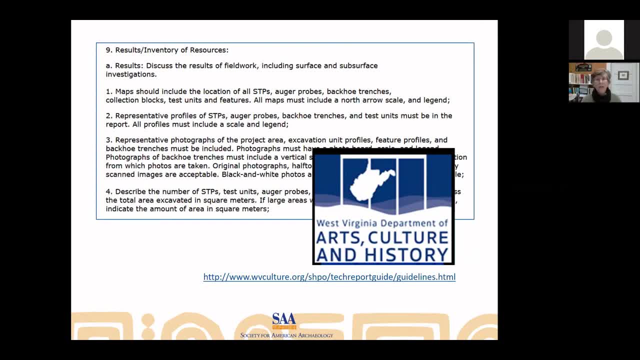 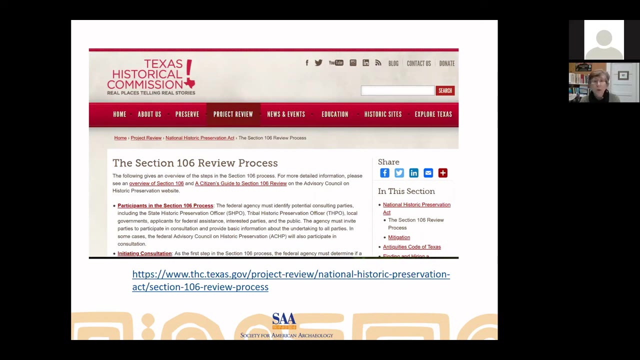 and how reviewers expect technical reports to be organized and formatted. You don't need to reinvent the wheel. The blueprint is already laid out there for you and oftentimes very specifically. Familiarize yourself with the SHPO's and the TIPO's in the state that you're working in. 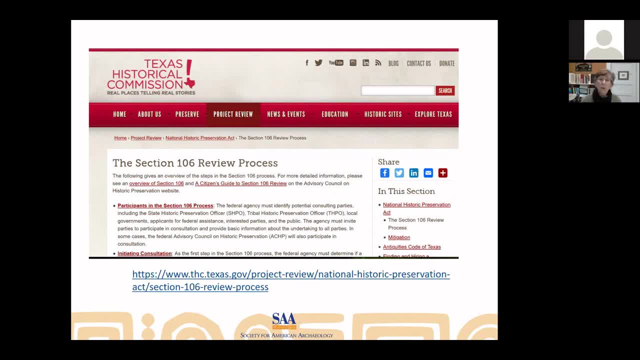 as well as who's responsible for Section 106 review. The process is similar in states across the country, but it's helpful to know what the reviewers are looking for in your report. Some people are sticklers for having the right form, having the references in the right format. 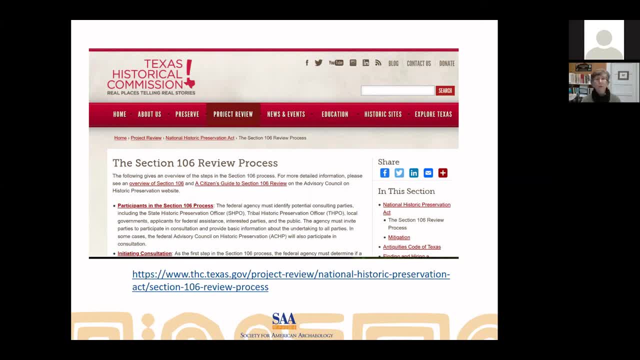 Others want to see that you're including information about why you ended your shovel test at a particular depth. So there are people reading your report. You have to take this into consideration too. Make sure you're familiar with the jargon. State websites are often very handy. 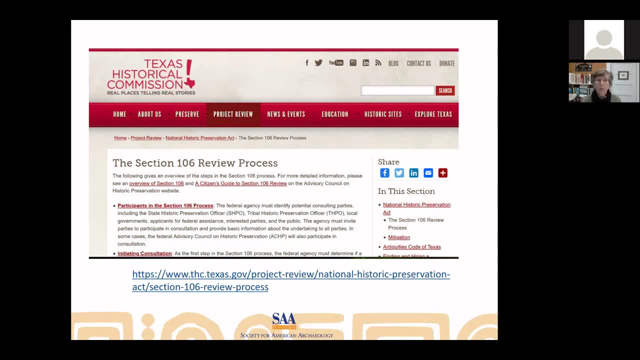 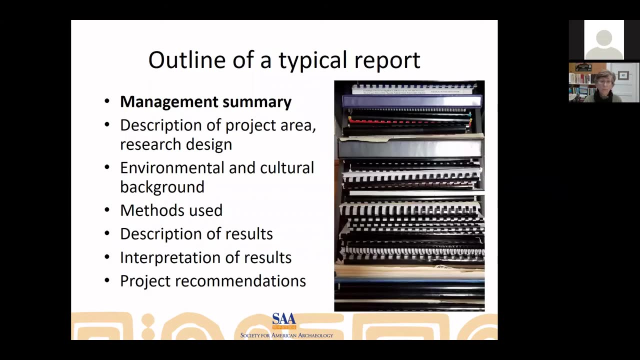 They have links to helpful resources to help you with your background research. They often include specifics about who manages them, who uses the state's archaeological site database, So take advantage of their work. So here's an outline of a typical report, And again, this is set out in those NPS standards. 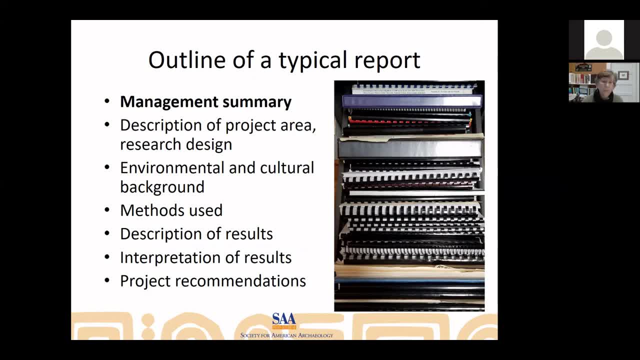 So what's usually in each of these sections? First, the abstract, or the management summary, gives a short overview of the project, the results and the recommendations. When you're writing, remember that this section is often read by people who are not professional archaeologists. 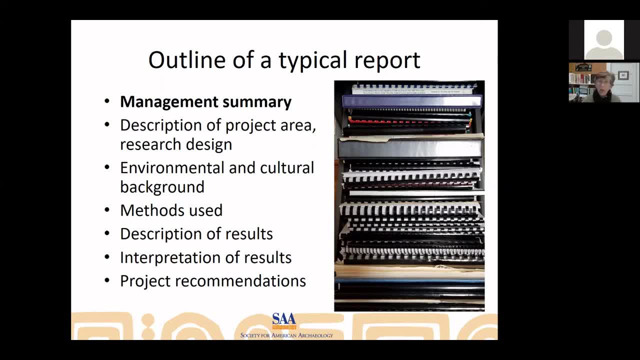 So what did you find And what do you recommend that they do about it? You have an introduction that includes a description of the project area or the area of potential effect: What agency requested the work, Who did the work and when. The project research design is outlined here. 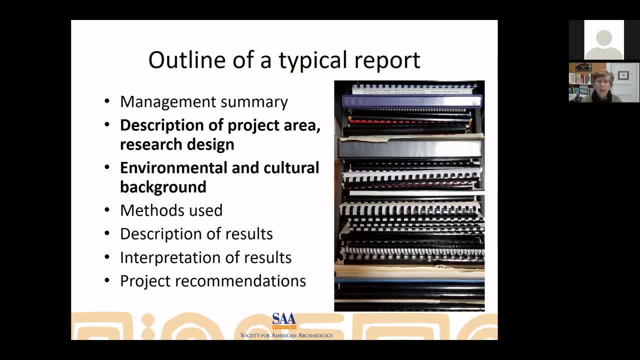 The research plan and the records and literature review in the background section should be done before the fieldwork starts because it guides your work. The background section provides an overview of the environment and the culture history of the project area and vicinity. Here you summarize the regional history both from archaeological work and from archival sources. 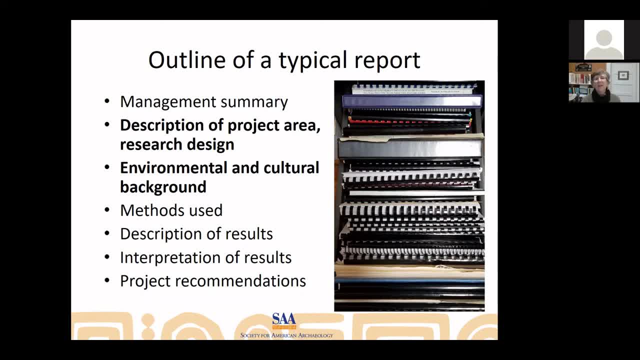 You are setting the scene for this project, this project you're reporting here. Typically you'll include previous archaeological research in the area. You'll include some mention of sites that have been listed on the National Register of Historic Places. Then you describe the field and lab methods that you used during the project. 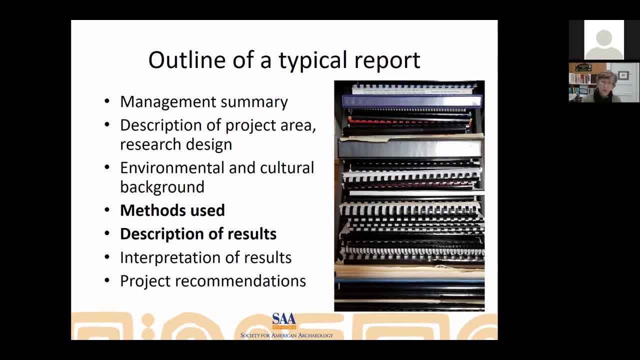 Including geophysical surveying, archaeological surveying, excavation, And then you present the results of your fieldwork and the lab analyses. This section is the real meat of the report. This section is where you include your maps. Talk about survey coverage. 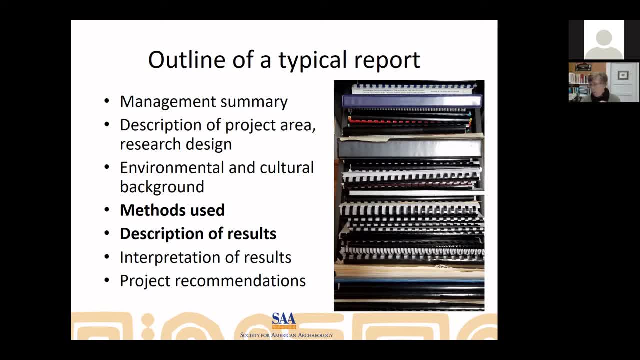 Talk about sampling procedures. You have- Sorry, You have- descriptions of newly recorded sites that you've discovered. You include- You include excavation profiles, Photographs, Feature descriptions. You You might talk about constraints on the fieldwork As well as talk about your artifact classification schemes and have descriptions of the artifacts. 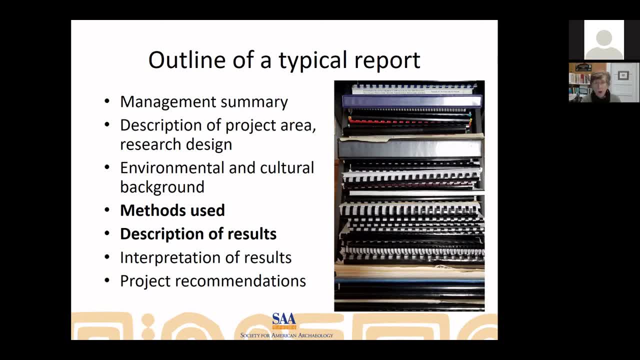 There will be results of radiocarbon dating and other specialized analyses in here too. Somewhere in here you know where the notes and collections will be curated. Finally, you'll have sections with your interpretations and recommendations. Are there sites that are eligible for the National Register based on your testing project? 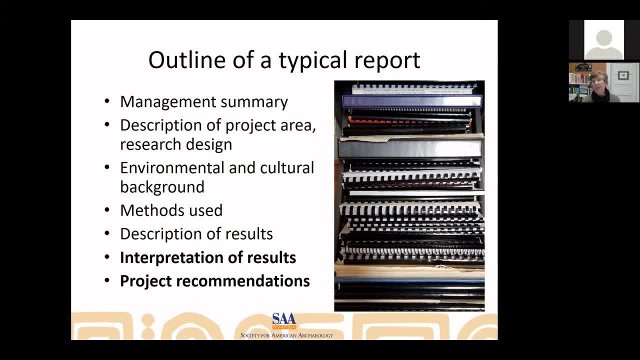 And why. If your survey did not locate any archaeological sites, why not? What are your recommendations in terms of further archaeological investigation Or avoidance of potentially eligible sites? These recommendations will go into your management summary at the beginning of the report as well. 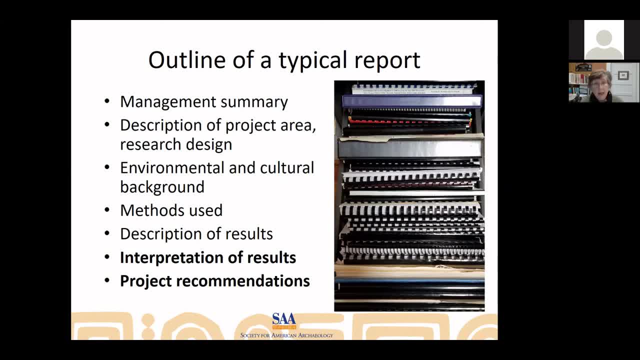 And then at the end you'll include references cited And typically you'll have an appendix that has maps that show site locations. In Arkansas, for example, the SHPO specifies that location, maps those quads with the dots on them. 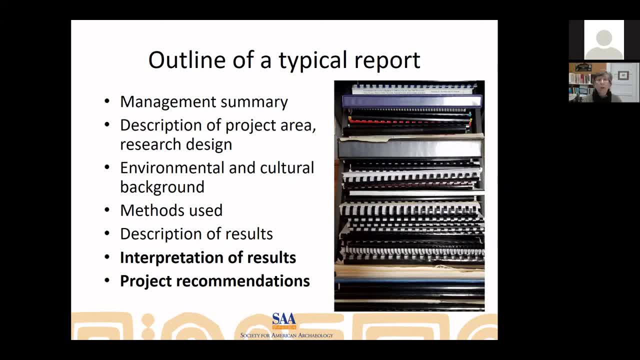 location maps should be separated in an appendix, marked not for public distribution, so as to protect the sites and the property owners too. So again, expectations for the outline and the contents of archaeological technical reports have been published by the National Park Service and included in various state plans and guidelines. 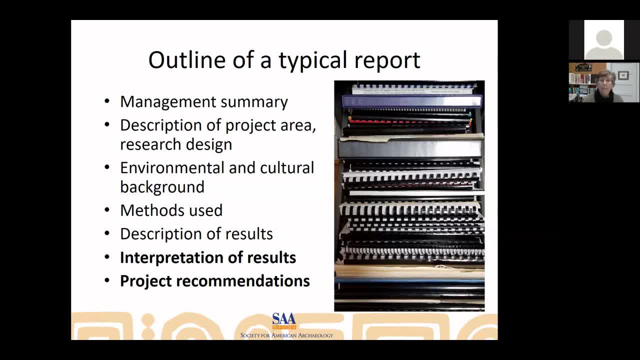 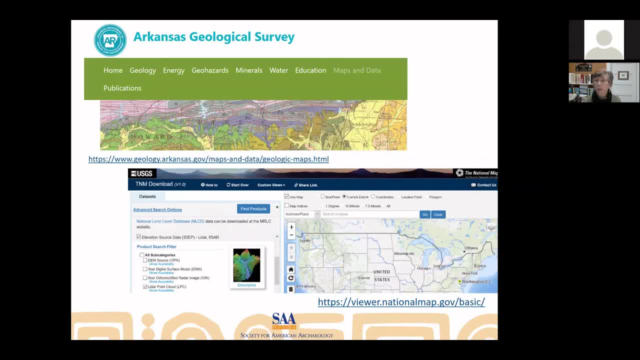 So find the one for your state and follow it. There are many resources out there to help you with your background research And, again, this is typically done before you go out in the field. but these resources are also important for report writing In terms of local environment, for example. state geological agencies typically publish geological maps and other detailed maps. 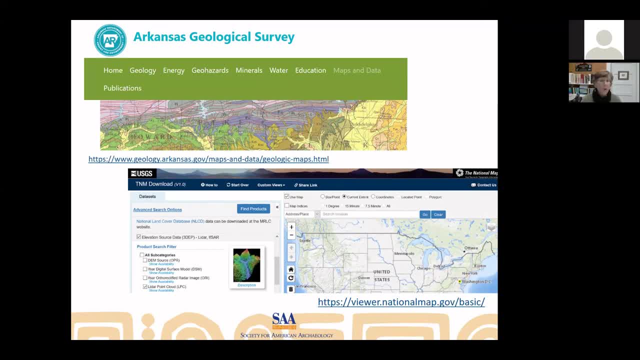 I work here in Arkansas. I want to know where the project area is in relation to the Arkansas nevaculate formation, because nevaculate was an important toolstone in and near the Washtenaw Mountains. So how close is my project area to the quarries? 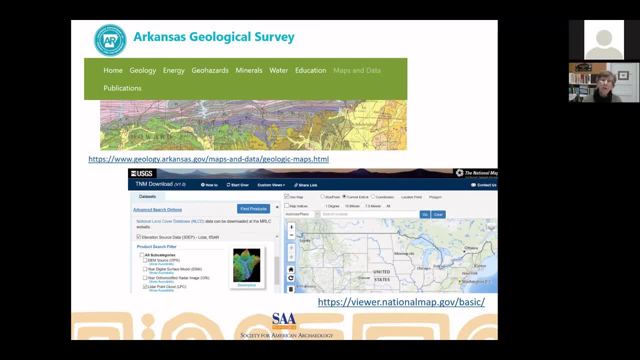 LiDAR data can be downloaded from the US Geological Survey and used to create detailed views of topography. More and more we're looking to see what's there before going into the field. This spring, I was getting photographs and even a video tour by email from a landowner and I was able to get the LiDAR. look at the LiDAR to see the earthworks that he was talking about. 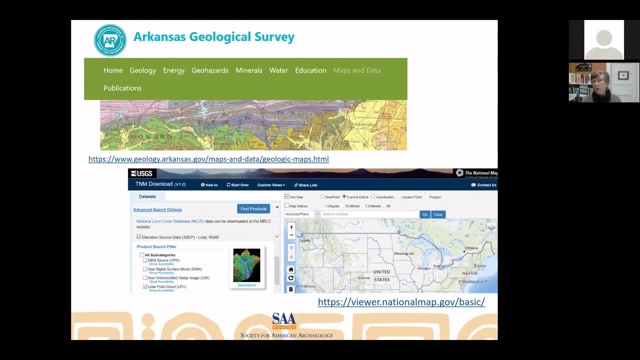 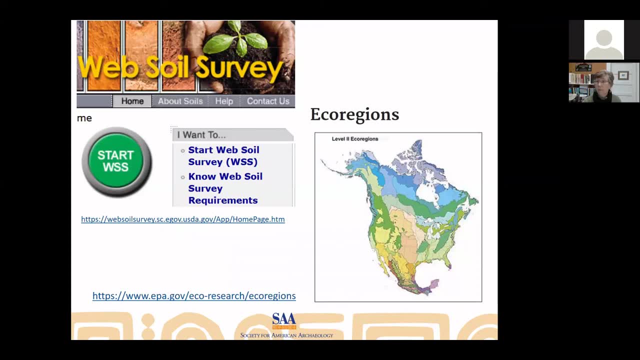 I could practically get the information to record the site without even setting foot on it. You can get soils information from the USDA Natural Resources Conservation Services Web Soil Survey. This updates the previously published Soil Conservation Services County Soils books. The US Environmental Protection Agency developed ecological region descriptions. 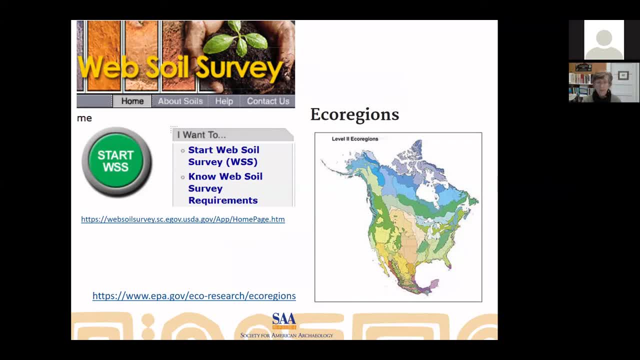 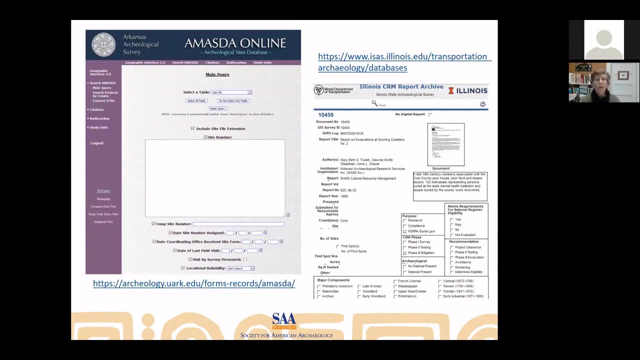 For North America and for individual states, And I find these very handy for my environmental background. What other archaeological sites and historic properties have been recorded in and near the project area? States maintain the archaeological site file databases, And access and search procedures vary state by state. 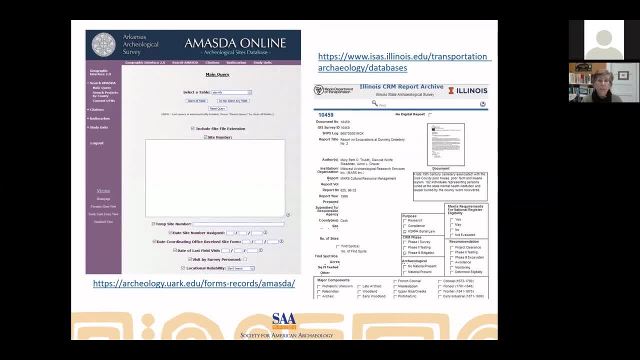 As you know, the site forms themselves differ state by state. Some states have multiple page forms. Other states have two sides of a five by seven cart. So there's a lot of variation here, But the states maintain these databases. Many states also have databases of reports and publications. 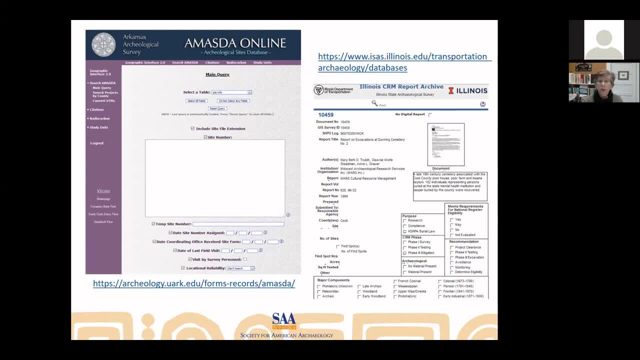 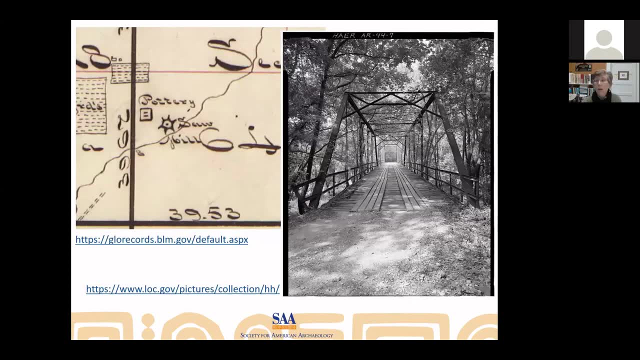 So there are digital versions of old reports that are accessible for download. You can search land patents and general land office surveys. Here we've got a pottery kiln and a sawmill located on the mid 19th century. GLO Historical quadrangle maps are available from the US Geological Survey. 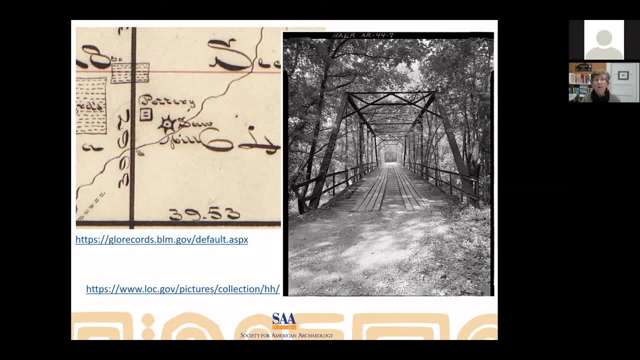 Oftentimes those historical quads have mounds located on them that aren't showing up on the modern ones. The Library of Congress makes available the Habs-Hare records, That's, the records from the Historic American Building Survey that began in the 1930s. 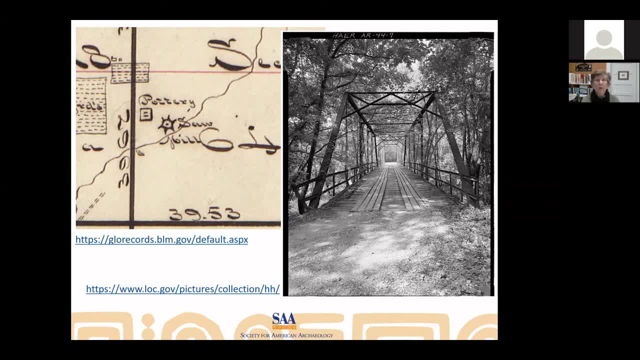 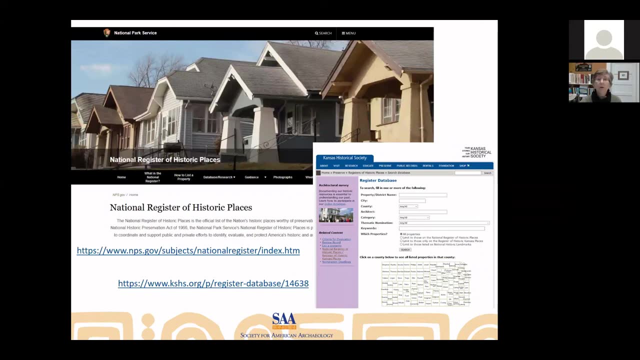 And later on the Historic American Engineering Record and the Historic American Landscape Survey. So if I'm recording a historic bridge, that's my go-to source. The National Park Service maintains the National Register of the Historic Places, And individual states often have web-based searchable databases. 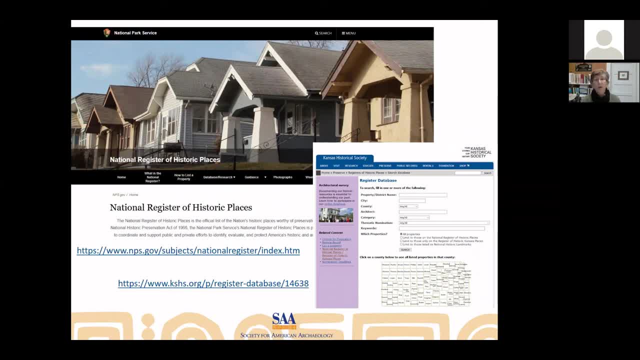 with listings for both national and state-level properties. So access is restricted to archaeological site file databases to protect sites, to protect site locations. But many of these other historical records are readily available via the internet. These are resources that you examined before going into the field. 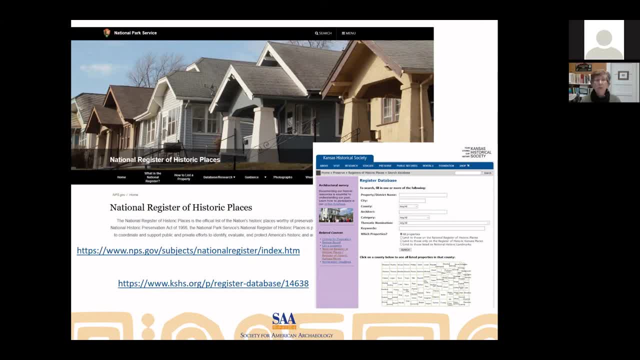 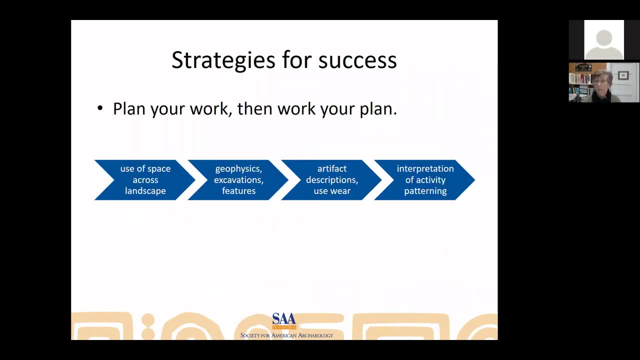 but they also inform the background research section of your report. Alright, so in addition to looking at these research resources, let's talk about some strategies for successful technical report writing. First, develop the project research design or research plan early. The research plan, the research questions, influence your field methodology. 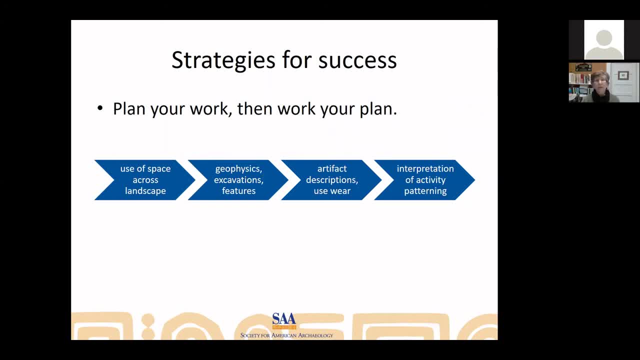 as well as the methods for artifact analysis. The ways that you record attributes during lab work may affect your ability to answer certain questions later on, So it's important to think. this process through first Changing the plan midway is not productive. You might have some discussion of constraints or problems encountered during the project. 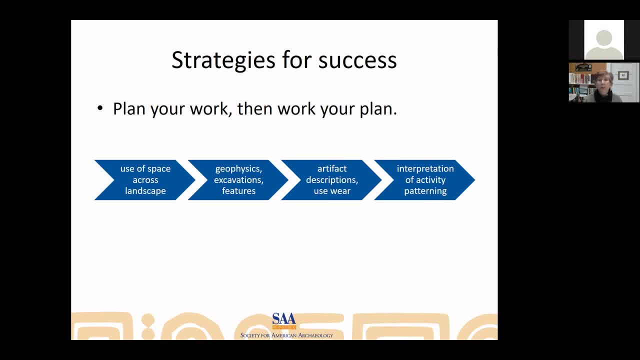 That might be important to have in there, but you don't want to just change course halfway through. In some cases, you're going to be asked to write a research design and a scope of work or a proposed plan for testing as part of phase two evaluation or conducting. 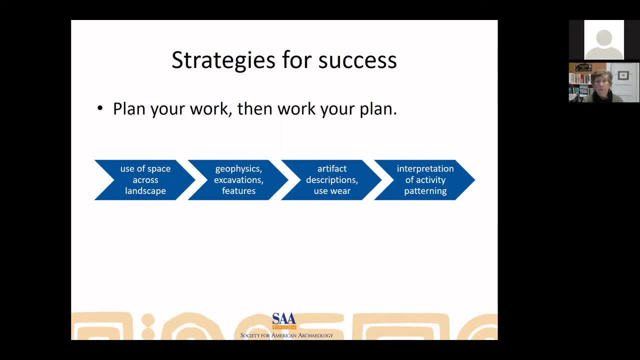 or as part of phase three, data recovery, before you conduct excavations. Not only does you and your firm have to calculate budgets based on the extent of the work you have planned, but the lead agency will want to see a comprehensive plan and how likely it is that your team will be able to carry it out. 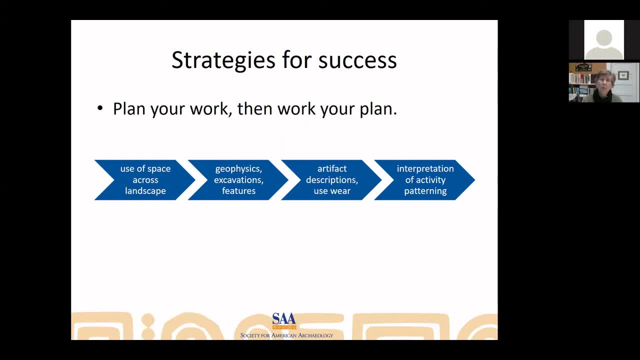 So what's been done before in the area in terms of research? What are the key questions discussed in the literature? You want to pay attention not only to previous CRM reports, but also to journal articles reporting current research. Be up on the current trends. 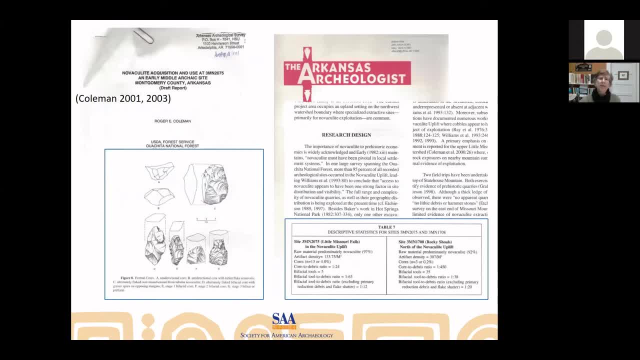 You know, as I've been putting together this seminar, I've been thinking about good reports that I've read and used in the past. One thing they have in common is they are formed around an engaging research plan. So here's an example. 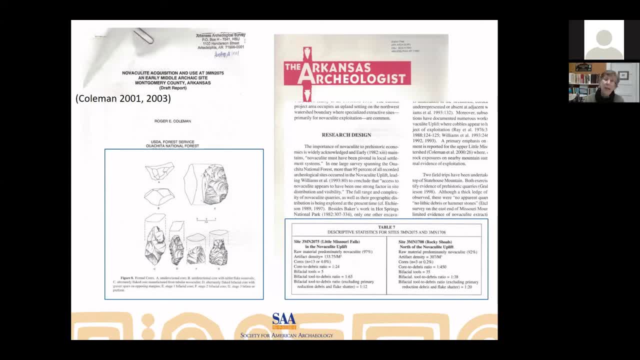 This is Nevaculate Acquisition and Use at 3MN2075, an early middle archaic site, Montgomery County, Arkansas. This one's by Roger Coleman, US Forest Service, Ouachita National Forest. Coleman tested a site on the Ouachita National Forest. 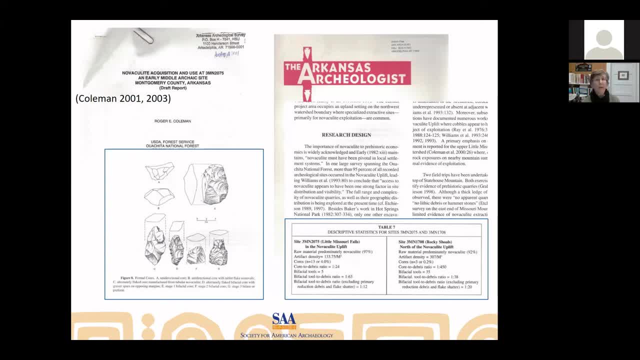 and recovered only 288 artifacts, 98% of which were in the form of lithic chipping debris. Now, this is not that many artifacts, especially since we're talking about a lithic workshop in the Nevaculate uplift, But what made this an interesting and useful report for me? 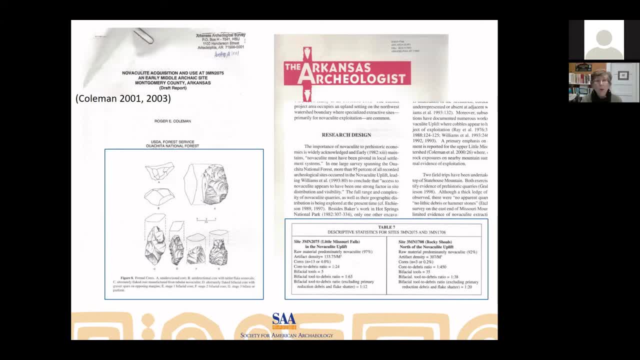 and later a journal article, is that he situated his analysis in a technological organization framework. He analyzed the site and its artifacts in terms of mobility, tool, stone acquisition, tool making and curation. He compared the results of this site to another one located outside the Nevaculate source zone. 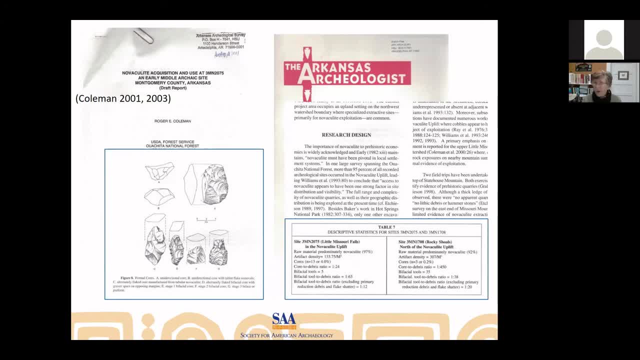 And he concluded that people at both sites were using a curated technology. They were relying on bifacial cores and tools, despite differences in the local availability of tool stone. Now, in the end, Coleman didn't consider Site 3MN2075 to be eligible for National Register nomination. 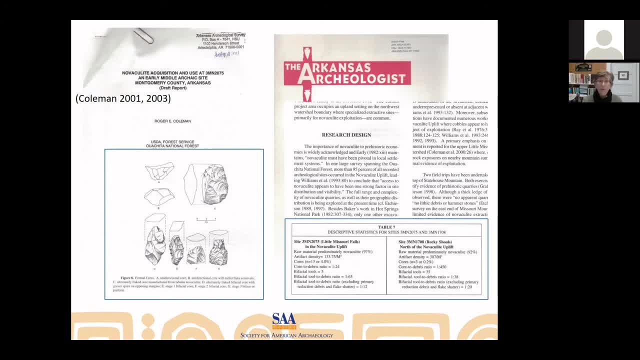 but he certainly got a lot of information out of the testing project there. I've come back to his report and the article a number of times because it starts with a research design. It lays out what to expect based on two alternative models. It offers a clear description of the excavations. 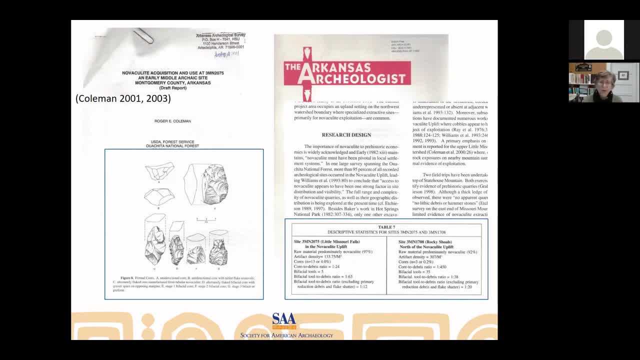 and the artifacts, and it structures the discussion in a way that invites further comparisons. So start with a research plan. This guides your fieldwork and your analysis, but it also guides your report. It makes for a more interesting and more useful report. 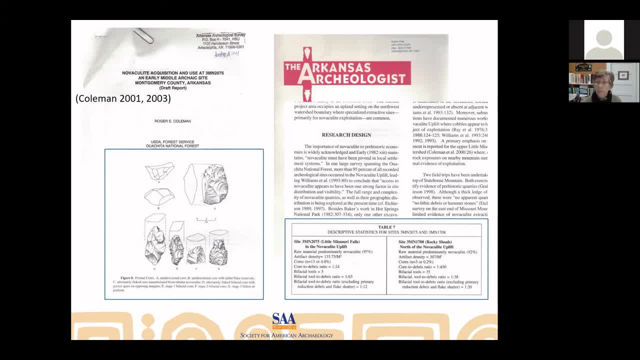 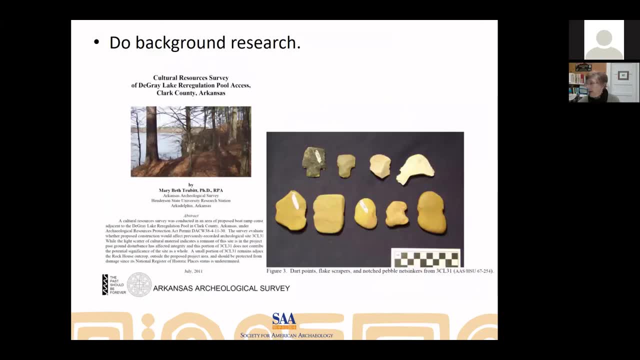 for people who are going to read it. Next, I suggest do your background research. Typically, you're going to look at what archaeological work has been done before and what has or has not been found at the site or in the area. You should do this before going in the field, of course. 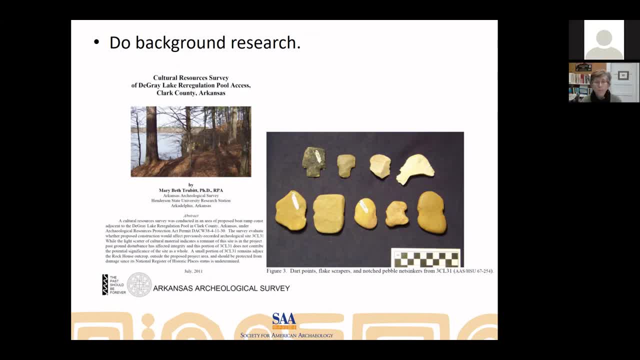 but it's also important for writing the report. Some years ago I did a little survey in an area of proposed boat ramp construction on a lake in Clark County, Arkansas. In preparation for the work, I pulled out the artifacts that we have curated here. 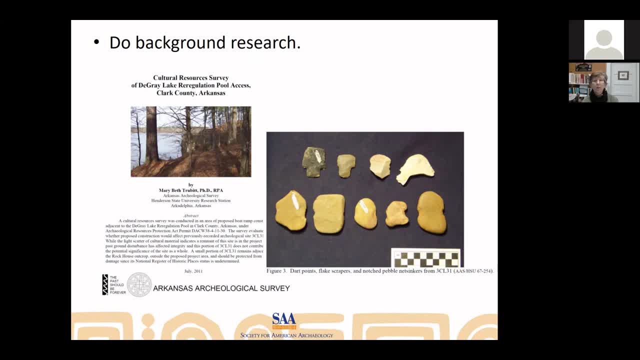 from a nearby site and I noticed that there were several notched pebble net weights or net sinkers in our collection. These are simple artifacts. They were used to weigh down fishing nets. There are middle archaic period diagnostics in this area. 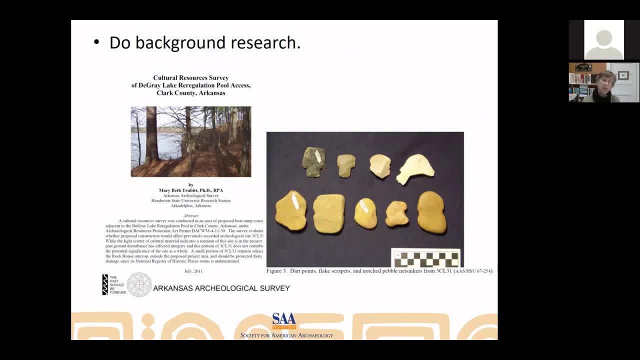 While I was doing shovel testing out there, I often saw folks in boats fishing just offshore And I thought it was remarkable that this place had been a good fishing spot for 8,000 years. This little detail made the project come alive for me. 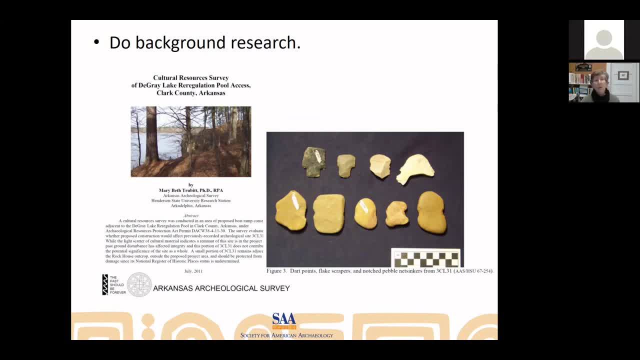 It created a link between the past and the present. It made it an interesting project For me. it made it more fun to write the report And hopefully I think it made it for a more stimulating report for the reader too. I think doing background research is especially important. 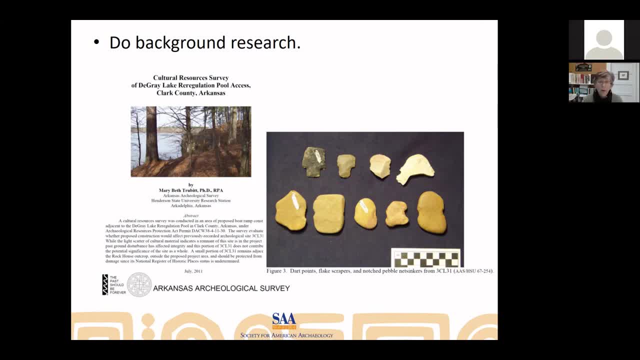 if you're working in a new area. I find that here in Arkansas more and more CRM companies are based outside of the state but doing work here in the state. So you want to know. for example, is there local archaeological evidence for domesticated plant use? 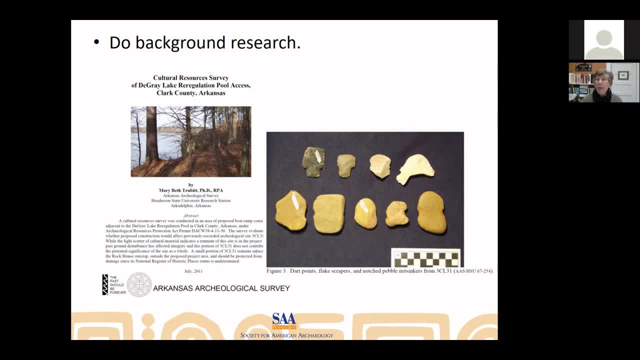 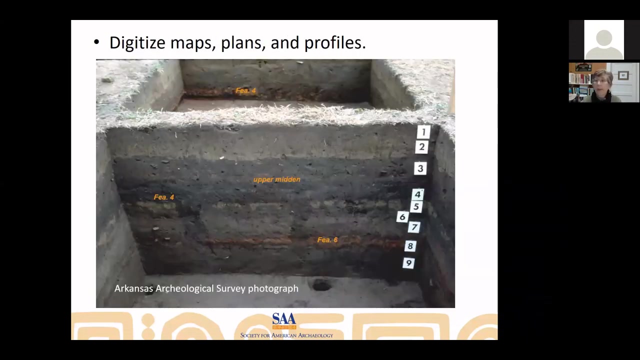 and when does that occur? You may end up finding charred seeds on your project that push that date back, that earliest domestication date back further in time, And that gives your project and your report even more significance. So you have to do that background research. 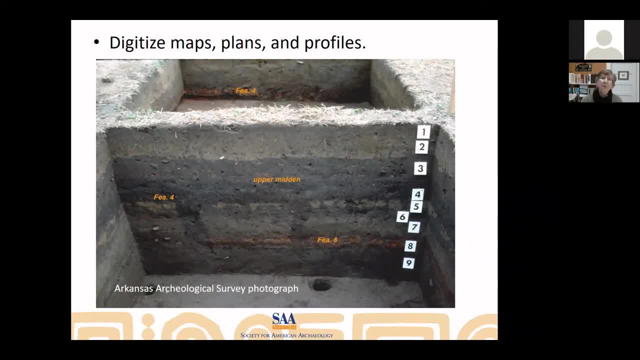 Next, I suggest that you examine maps and excavation plans and profiles. Take the opportunity to familiarize yourself with the spatial layouts. I always start with maps and profiles, I think spatially. I want to look at it spatially. How many units were excavated? 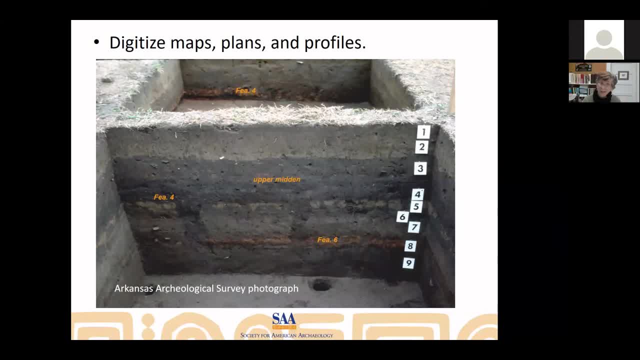 Where were they placed? What's the stratigraphy look like? What's the sequence of constructions at the site? I find for me, drawing or digitizing excavation profiles is an important way to understand and then be able to describe the site's stratigraphy. 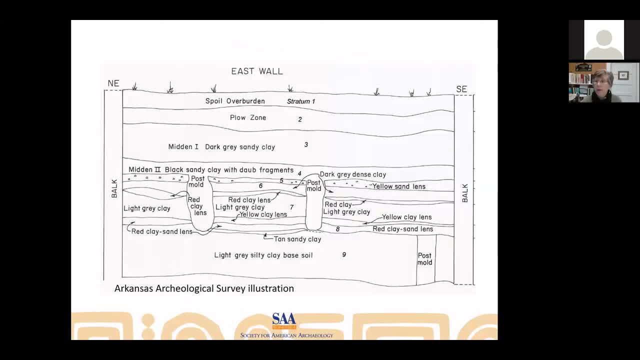 Now I know that recent trends in CRM emphasize specialization. The field director may not be the drafts person, may not be the artifact analysis, may not be the author of the technical report, But I find examining maps and profiles is key to understanding the site layout. 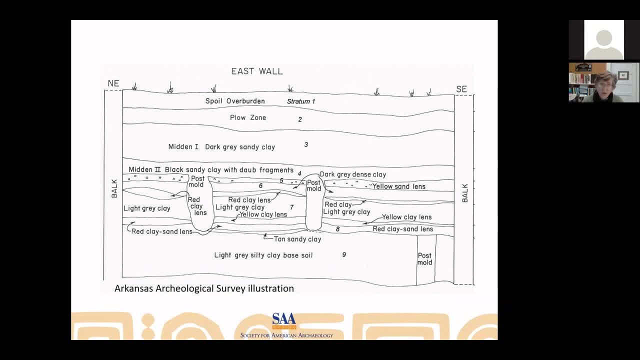 key to understanding the stratigraphy, And this is especially true if you're not in the field, If you're working with a legacy project. this particular profile comes from an early 1970s project. I wasn't here then, So it really helps you work things out. 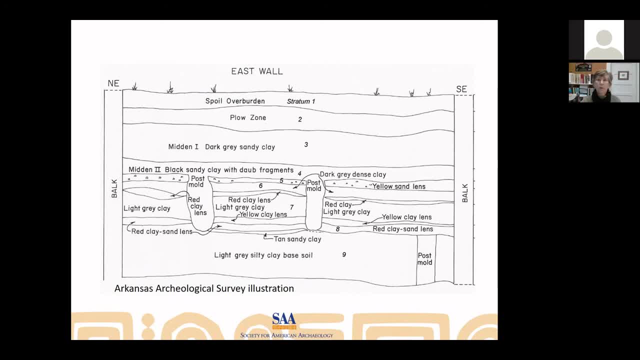 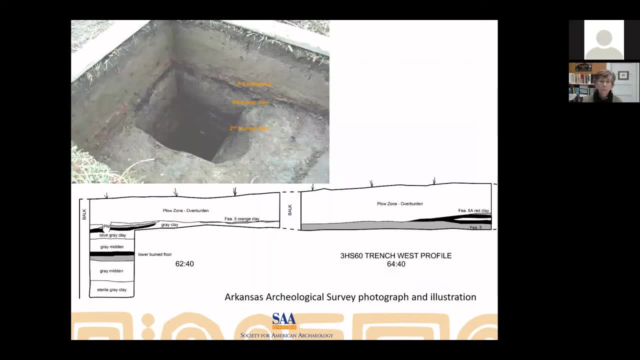 After formulating the research plan and doing the background research and doing the field work. that's where I start. It's also a reminder of how important, accurate and complete field records are to the final product, Once you try to assemble field drawings into illustrations for your report. 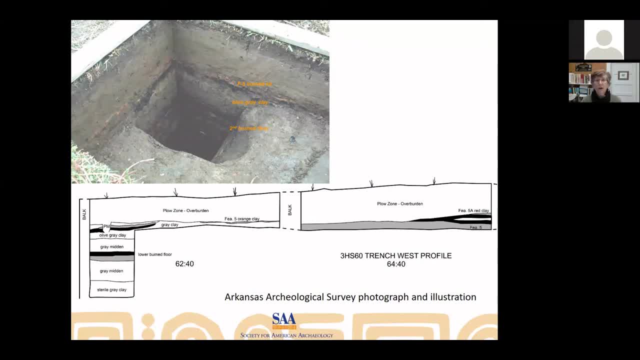 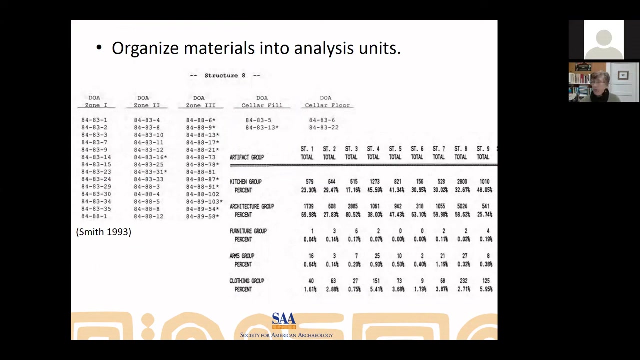 you really get an appreciation for accurate field drawings. You appreciate it when the soil descriptions and the profile drawings match up at corners or match up on either side of the box. Then I turn to generating tables. My next strategy is to organize excavated materials. 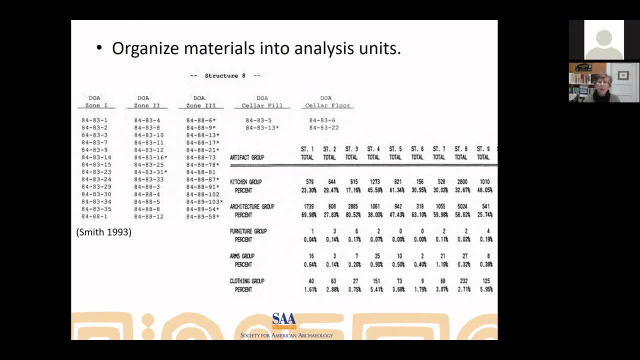 into analysis units. Here we can use strata, We can use features or clusters of features, We can use sites. But we are organizing the material into analysis units so that we can then make comparisons. Here I pulled up an example from a federal period fort in East Tennessee. 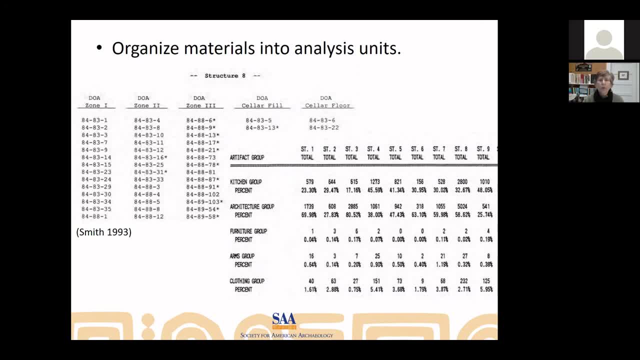 The analysis units were depositional zones within excavated structures. We listed which lots or bags came from each zone. For some purposes, the analysis units for each structure were combined so we could compare one structure to another. Details are important. You have to make sure your numbers 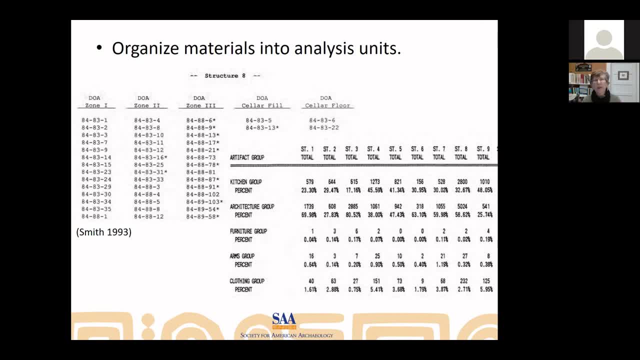 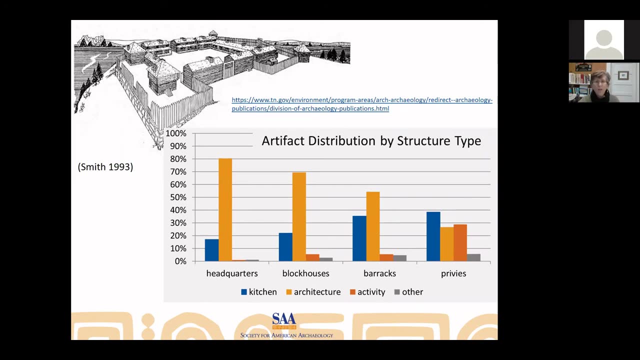 add up in your tables. You have to cross-check between tables. Mistakes and inconsistencies make your reader doubt other aspects of your work as well. So details are important, But you have to be able to refocus on the big picture when it comes time to write the report. 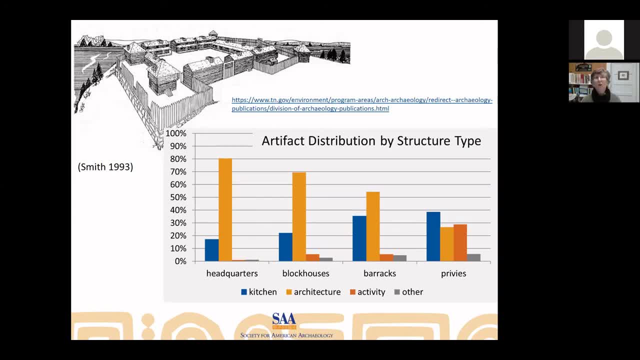 So to make and interpret meaningful comparisons you need to use analysis units. So at Fort Southwest Point in Tennessee, for example, we inferred different functions to the different structures based in part on the artifacts found in them, And here we can see that the headquarters 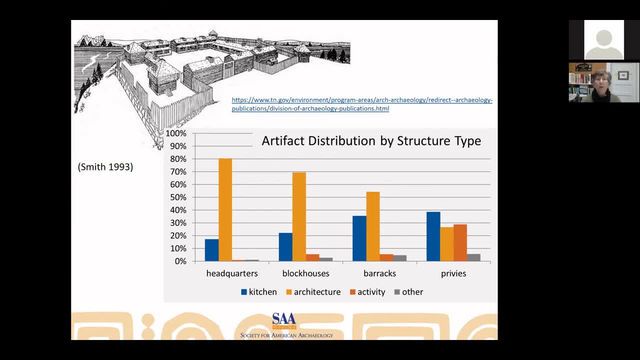 or the administration building, and the block houses at each corner of the fort had lots of architectural artifacts. The barracks where soldiers lived had more kitchen-related artifacts And the privies had even more dishes and glassware, as well as a lot of activity-related artifacts. 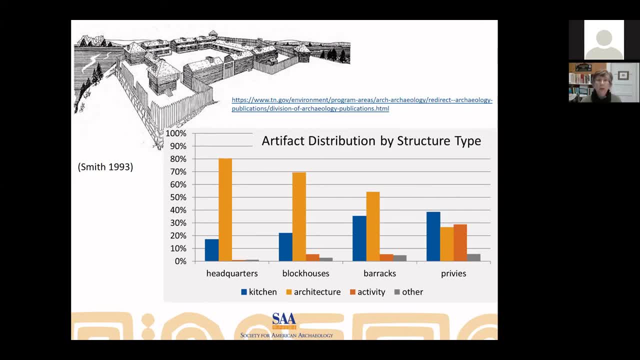 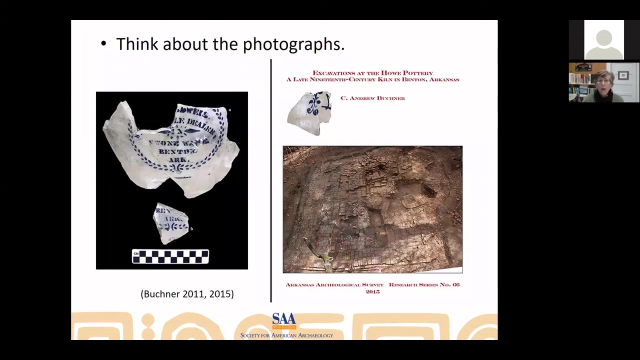 and more of the minor categories like clothing items and buttons. So you have to be able to go between the specific proveniences and the larger analysis units in order to make your interpretations of the whole thing. Another suggestion that I have is to keep the future illustrations in mind. 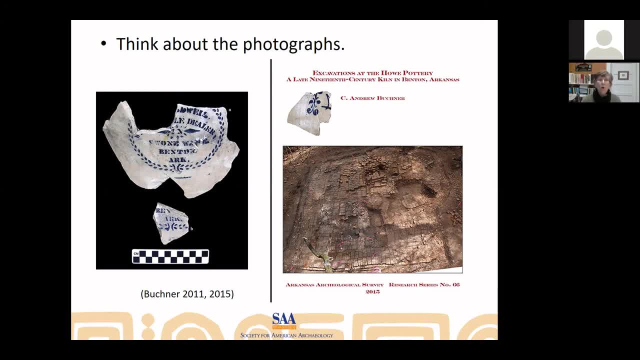 when you're photographing in the field or when you're illustrating sets of representative artifacts from survey or excavation. Remember that field photographs are what you have to show people. after it's all done, It's worthwhile to take the time to clean up and declutter the frame. 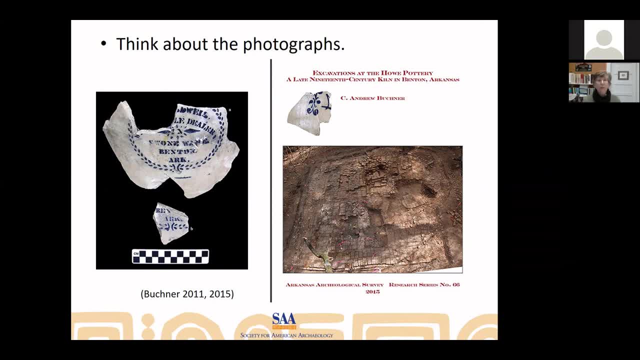 Think about lighting and shadows. Set up your shots In the lab. think about how you want to lay out artifacts for illustration or how you're going to ask the photographer to do this. Are you going to group artifacts by provenience? Are you going to group artifacts by type? 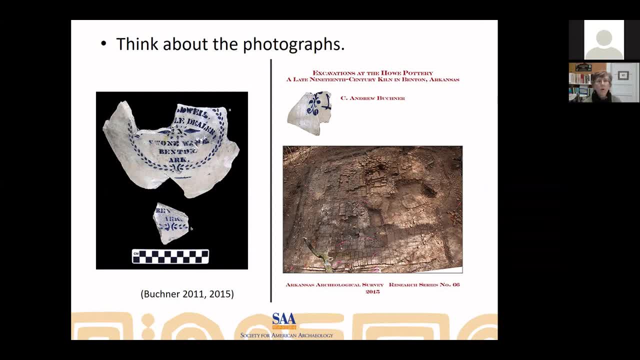 How are you going to do this? Think about the caption that you'll be writing and what you're describing that you'll need to show in a figure Again, adequate documentation in the field and in the lab, using sign boards, using photo logs. 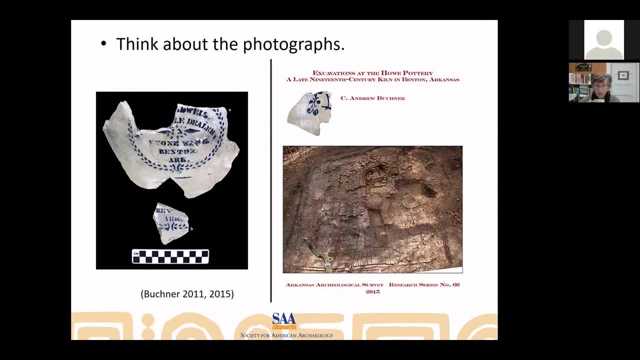 will make report preparation more efficient. later on. You may not want to, you may not be able to Go back to the artifacts Earlier this year, when I was writing at my home office and I really appreciated having complete photo logs on the server so that I could write the captions. 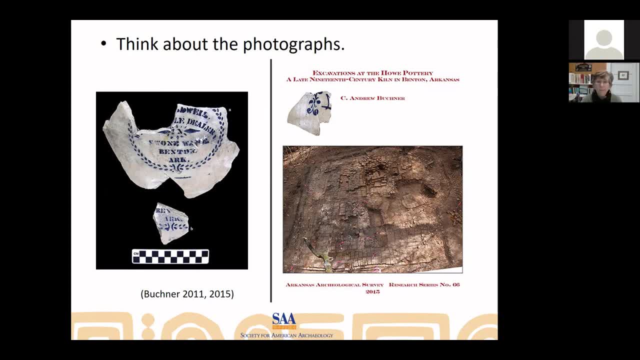 for the illustrations. I didn't have access to the lab at the time. This particular publication began as a report by Drew Buckner, Pan American Consultants, And his report presented the results of phase three excavations at a stoneware pottery kiln site. 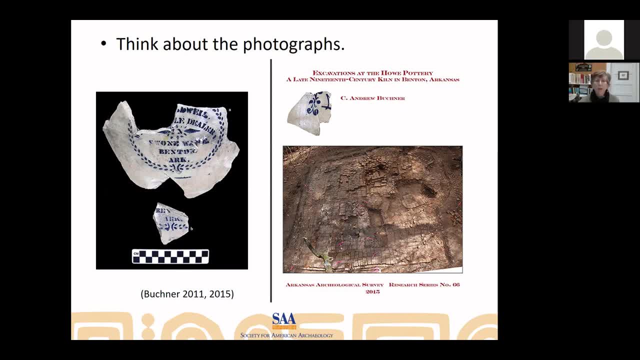 that was in the path of road widening in Benton, Arkansas. In addition to the excavations that were done, in addition to the excellent photographs of the superimposed kiln structures, there was a circular kiln for firing stoneware and, later on, 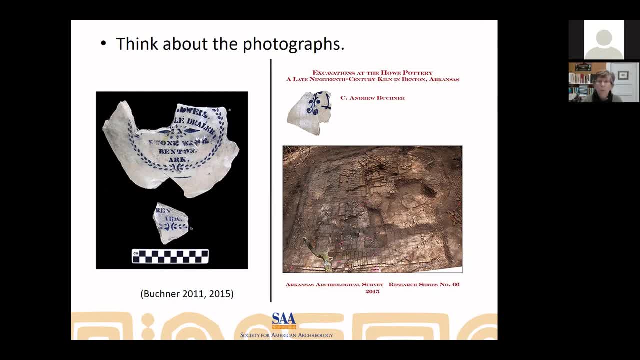 a rectangular kiln that was made to produce bricks. The report also has excellent photographs of the sherds that were recovered at the site. The report also has an extensive background section that brings together available archival information about the pottery industry in Benton during the late 1800s. 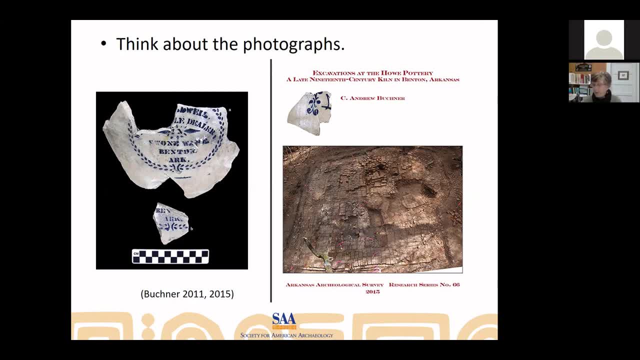 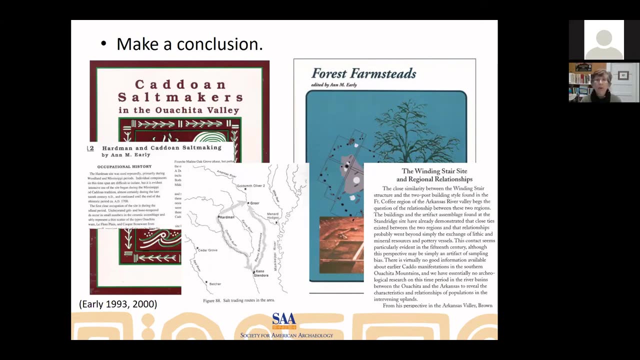 and includes historical photographs as well. So this was an interesting report. It wasn't boilerplate. Finally, you want to bring it all together in the conclusion section of your report. If you think about the structure of the report, it often goes from: 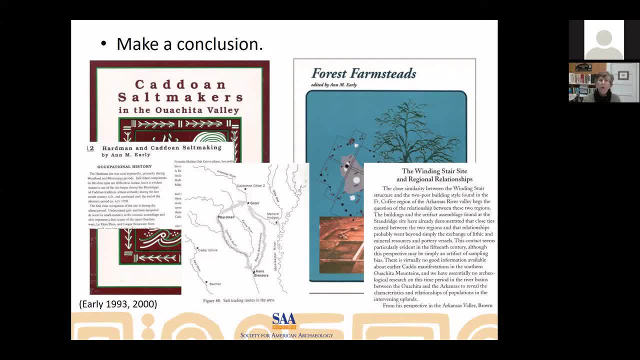 broad and general, with your background sections, to very specific with your methods and your results sections. But then you need to broaden back out again in the conclusion. Sometimes this means putting the pieces back together to discuss temporal trends and summarize the components or the occupations at the site or the sites. 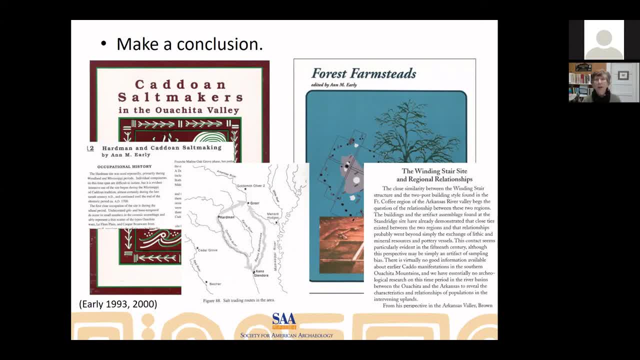 It's important to include ways or technology or architecture and community patterning as revealed by your archaeological investigations. I think the conclusion should not just summarize what you've done, but emphasize what was important about the project, what we've learned, why it's significant. 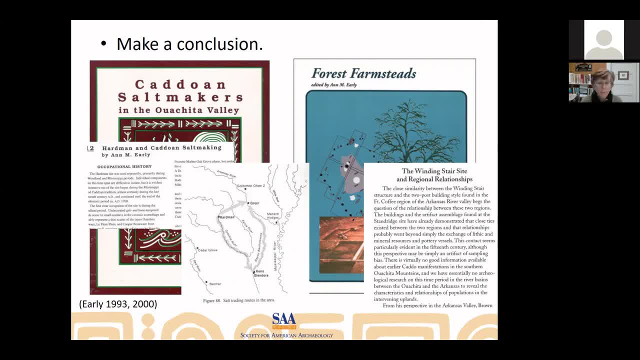 and where should we go from here? This would be in your perspective. In these specific examples, Anne Early redefined the phase sequence for the middle Ouachita River Valley over the last millennium. She linked salt production at the specific site with the regional trade in salt. 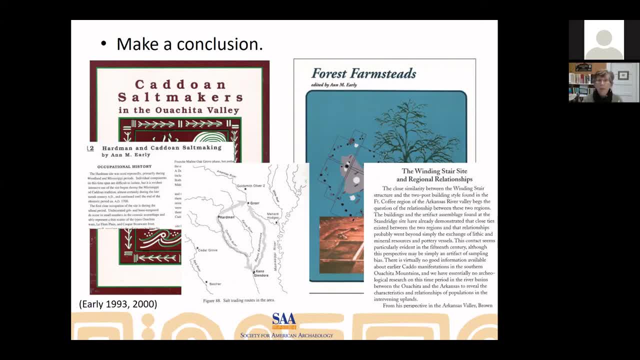 She tied site architecture and cultural patterns in the Ouachita Mountains to the broader region. What have we learned? Where do we go from here? Well, you say. these two examples are from the survey's research series. The authors had time to develop conclusions. 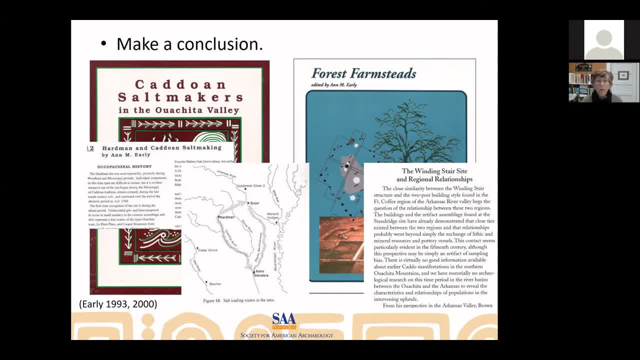 Yes, but these were technical reports before they were published in the research series. They were technical reports that ended up published because they made conclusions, because they were useful to the broader temporal and spatial regions And because of that they're useful to a broad audience. 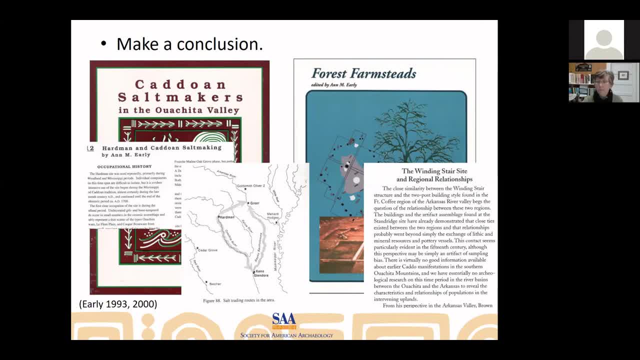 even 20 years later. A reviewer made a comment on my report manuscript recently that I needed to pay attention to the final paragraph because this is the last word on the topic. It's hard because by the last chapter you're tired, But they're right. 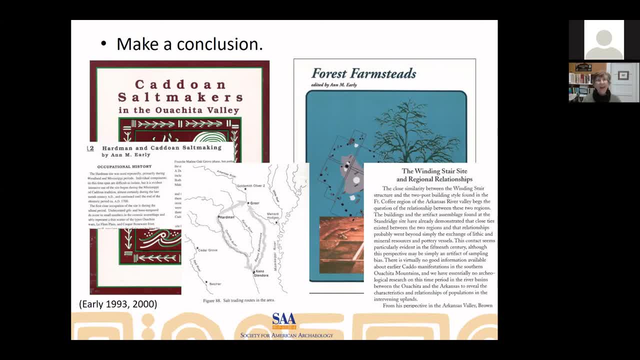 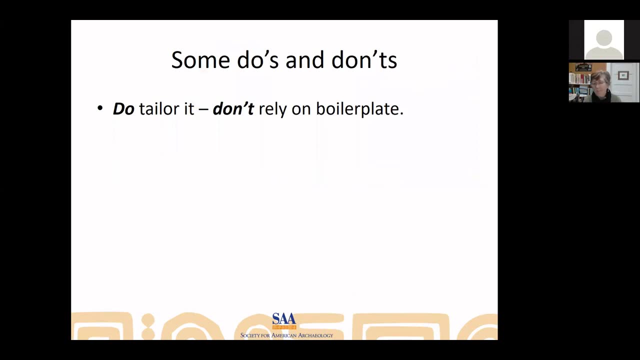 You need to end strong, And you should also remember that some readers may only read your concluding chapter, So pay a special attention to it. Alright, so this brings me to the final section of the seminar. I'm going to give you some do's and don'ts. 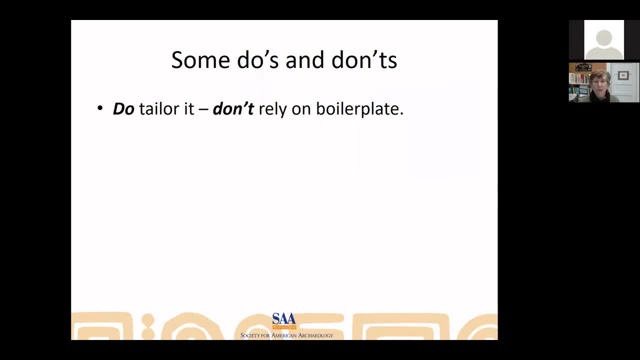 This is mainly based on things that irritate me when I'm reading technical reports. Tailor the background to the project area and to this specific project. Don't rely so much on boilerplate. The report outline has a set structure, but the text. 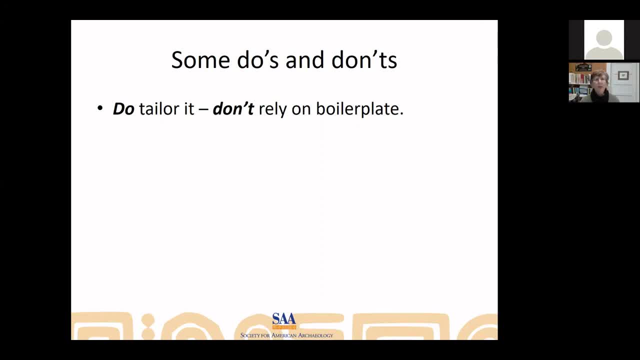 shouldn't be reused again and again and again. The literature review should include research that's appropriate to the area and the topics. I don't like to read boilerplate with the same references from the 80s and 90s. We're now in 2020.. 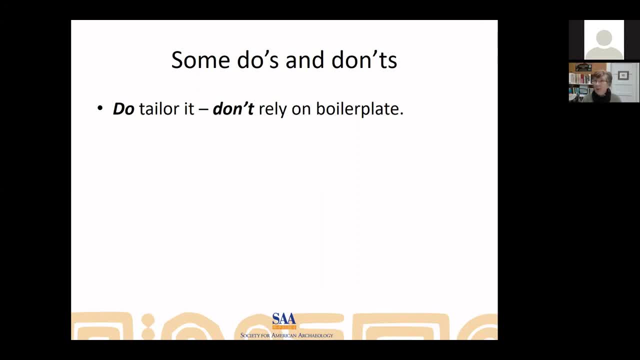 I don't like to read references to the wrong county. If you're going to use boilerplate, at least proofread it. Reviewing past work in the region sets the stage for comparisons and interpretations of the current work. This is really why you're including. 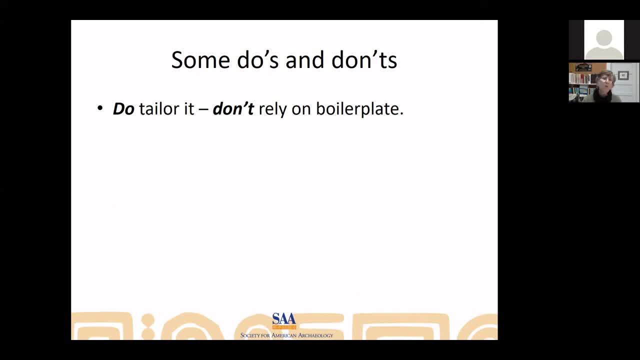 the information in the report in the first place. So you want to do it up front and save yourself the added work when you get to the final chapter. You should define your technical terms and don't rely too heavily on jargon. You can explain. 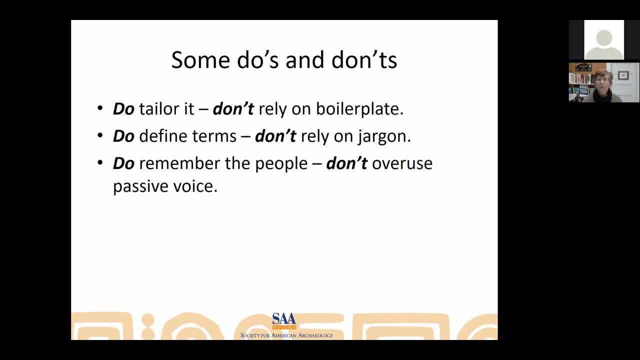 complex ideas using straightforward language, using straightforward sentence structure. Remember that there are people involved in this process, in the work, in the writing, and certainly the people who lived here in the past. Readers get tired of reading passive voice, But even more so. 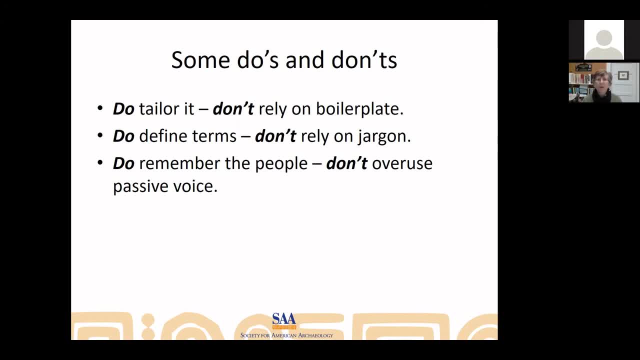 it tends to blanch the people out of the process. People lived at these sites. Archaeologists investigated these sites. You don't want to just kind of remove them from the picture. This can be tricky because I think a lot of us tend to emulate a. 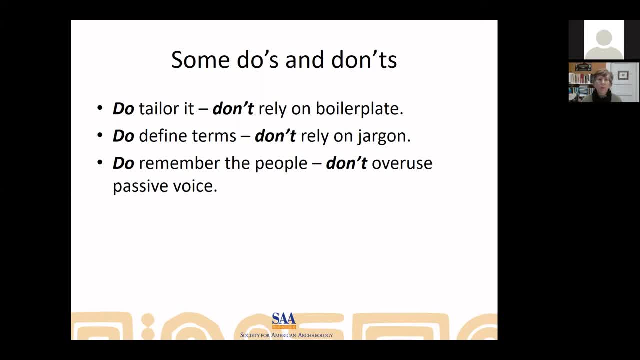 dispassionate, objective tone for technical reports, But too much passive voices is boring to write and it's boring to read And it reduces communities of people to sites and objects. Describe and illustrate archaeological sites and the methods that you use, but don't put specific. 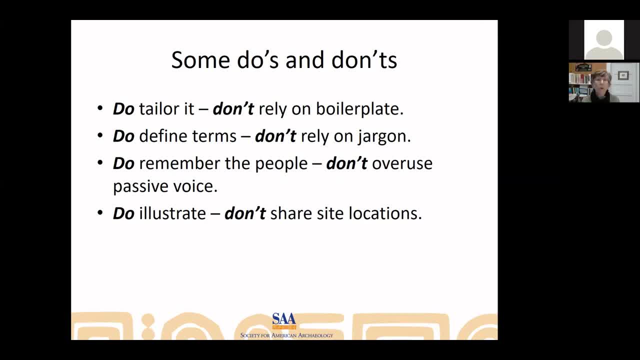 site locations and detailed location maps in the body of the report. Often site forms and location maps are included or separated out and put into an appendix that has a restricted distribution. I mentioned before. this is a requirement in Arkansas. Also think about it. 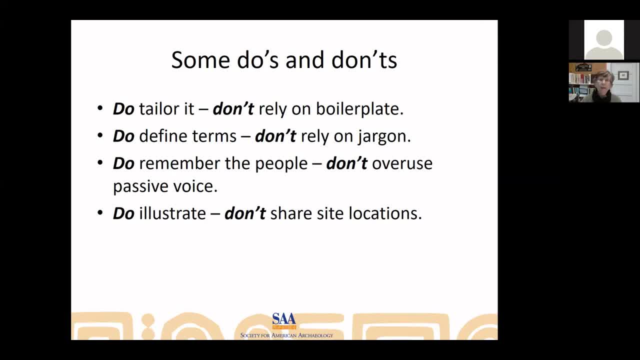 If your report is later made accessible online, you won't have to go through and black out certain figures if your detailed location maps are already separated out. I think it's a little ironic that as we get better technology for generating detailed maps for making our reports accessible, 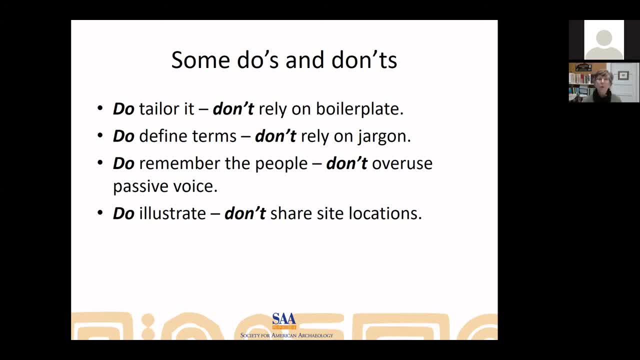 to wider audiences. we have to think harder about what not to illustrate and share. Lately I've included detailed LIDAR maps in the site form. I put them into the site form rather than publishing them in an article to keep from oversharing the site location. 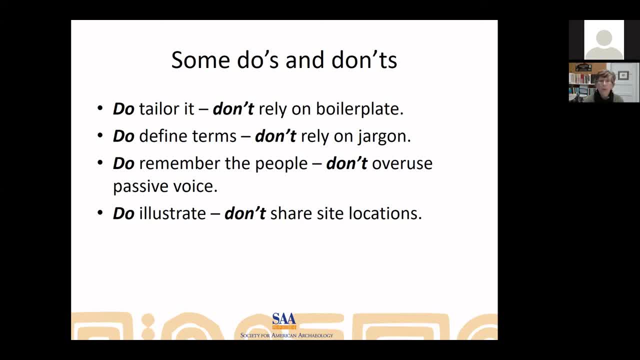 and risk trespassers and looters coming to the site. You may also need to pay attention to avoid photographing or illustrating human remains or mortuary objects, So not everything has to be shared with everyone. Adjust the length of the content of the report. 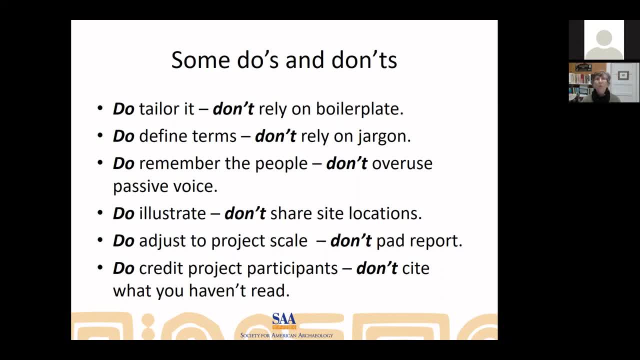 to the size and scope of the project. Don't fill a negative findings report with unnecessary details to make up for a lack of field effort. I've read many reports that are all set up and no delivery. You want to acknowledge and credit the project participants, People who 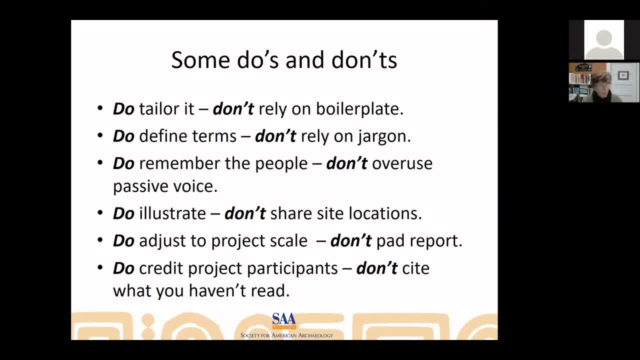 contributed to the report, people who made the maps and illustrations, and also published sources that you relied on for background. Don't cite sources you haven't read yourself. Add bibliographic information as you're writing. Don't make it a habit of saying, oh, I'll go back. 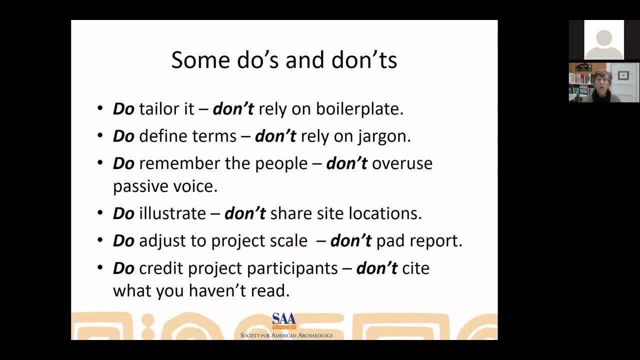 and add that in later on. Do it while you're using it. Do it while you're writing it. Familiarize yourself with the Society for American Archaeology style guide and get in the habit of using it. Yes, your office may have. 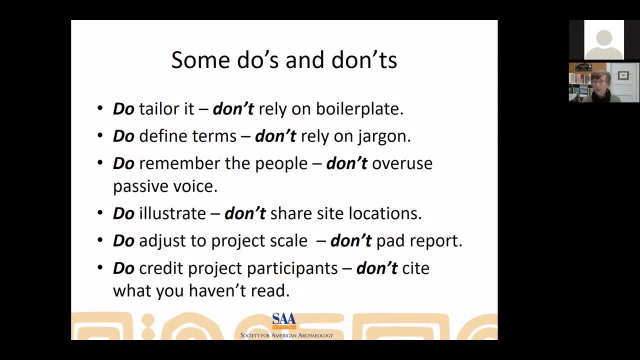 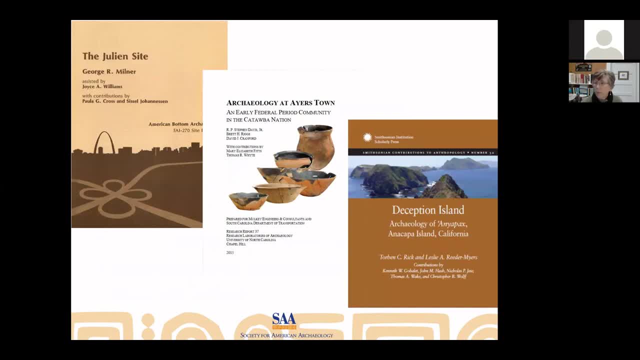 an editor, but it's time consuming. So get in the practice of doing it right the first time. You know. I agree that writing is hard. Sometimes it's hard to get the words to flow. It's like that for all of us. What I can recommend is to write every day, Write regularly, Get in the habit of writing. For me at least, it's easier when I'm in a schedule. I'm in a pattern of writing for a couple of hours every morning, or at least several times a week. 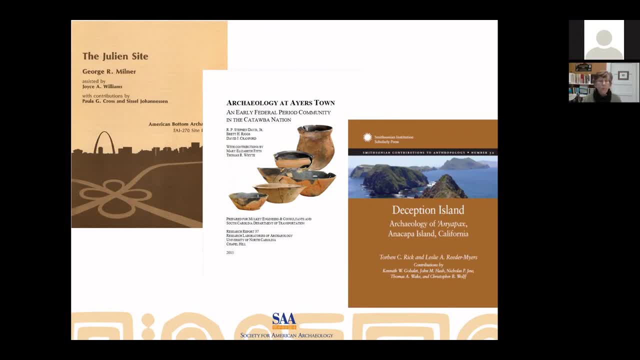 Writing's a matter of practice, so get in the habit of it. I read Mitch Allen and Rosemary Joyce's chapter on Communicating Archaeology And I like their recommendation. Here I'm quoting from them. I quote: Have fun writing and your readers. 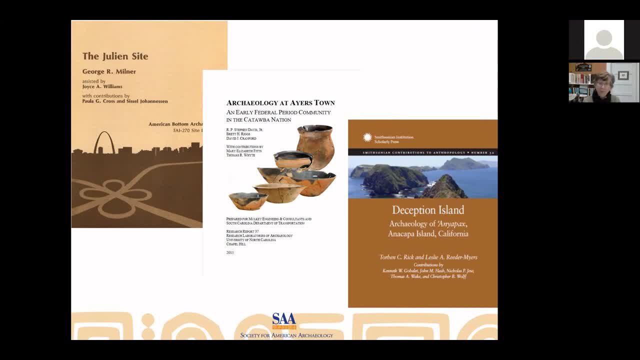 will have fun reading what you wrote. But whatever you do write, The more you do, the easier it gets. End quote. Finally, I'm going to make the suggestion that you read other archaeological reports. I put some readily accessible series on. 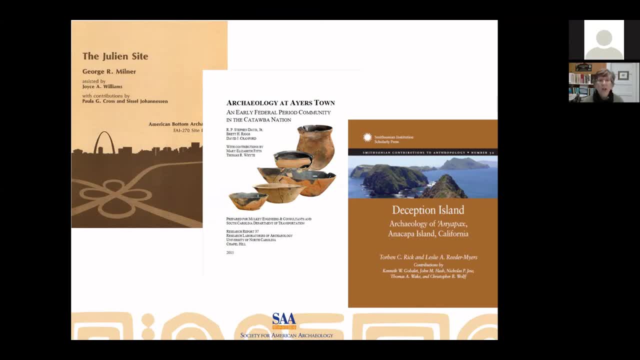 the handout for you, And I also suggest that you read outside the field of archaeology too. Read widely. Some archaeological writing is stodgy or dry, so it's helpful to have good writers that you're reading, so you have good role models. 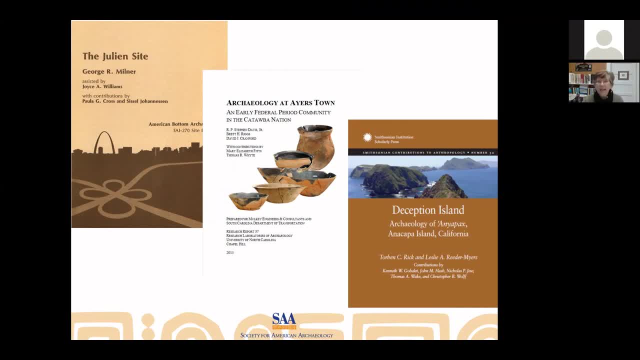 for writing that's interesting and engaging, And keep at it. Archaeology has many different aspects. You can write for part of the day, you can work on maps or artifacts part of the day and, before you know it, you'll be able to get that report done. 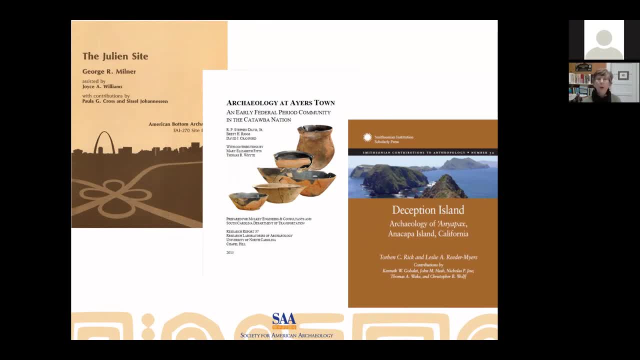 Then you have to have someone else read it and give you feedback. You have to remember that writing is communication. You need to learn whether your report is communicating what you intended it to communicate. Is it communicating what you intended to say to your audience? 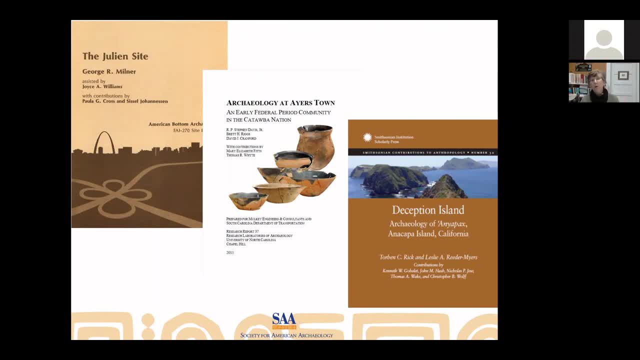 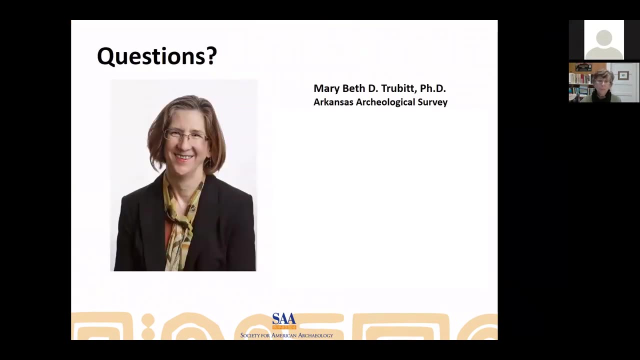 Get comments and feedback from others. Incorporate those as you make your revisions for your final version of your report. It's a process And keep at it. You can do it. So that's all I had. I am happy to answer any. 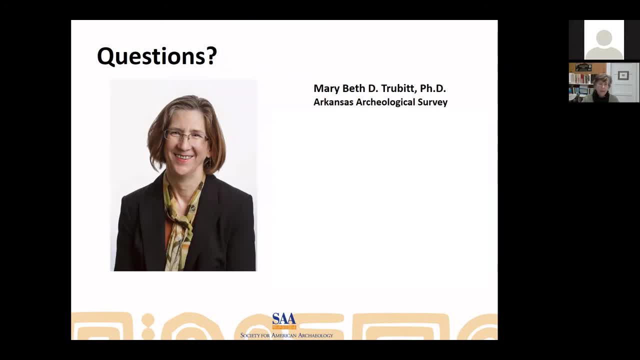 questions you have here. This is clearly a before times photograph here, But I also put my business card, so you have my contact information And I'm happy to answer any questions you have. If you want to type questions into the Q&A or into the chat, 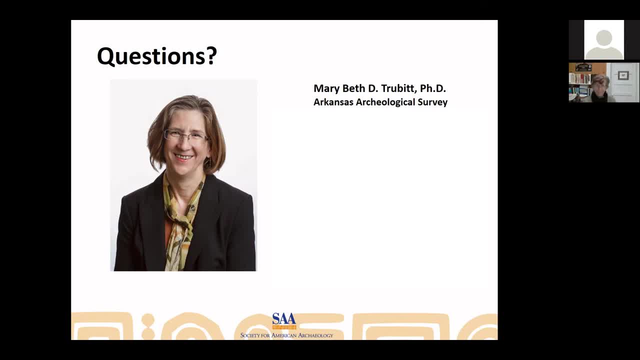 It can take a few minutes for people to type, So we'll just wait for a little bit. Alright, so we have a question: How should one handle gray literature in archaeological reports? You know, I hear a lot about gray literature. Well, you know. 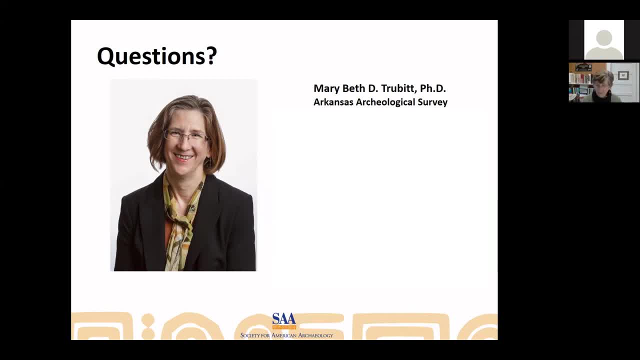 what we're talking about are reports that have a limited distribution, But they are out there And they are accessible. So first you have to find them, And your best source is going to be the, the SHPO's officer, Whoever in that state handles the. 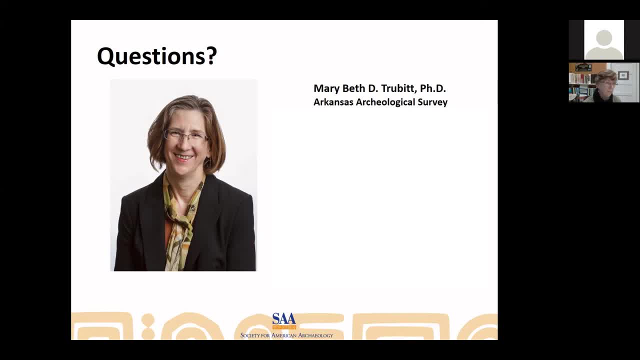 handles the archaeological site file database. Often times that same agency is going to have that database of archaeological reports, So you should be able to get- if you can get access to the site forms, you can get access to that database of archaeological reports. 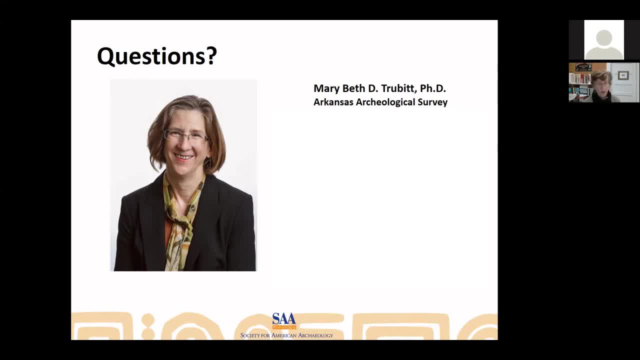 And often times you're able then to download a PDF of it. You know how do you include it. like anything else, Like anything published, How do you cite it? Take a look at the SAA style guide: 2018 version of the style guide. 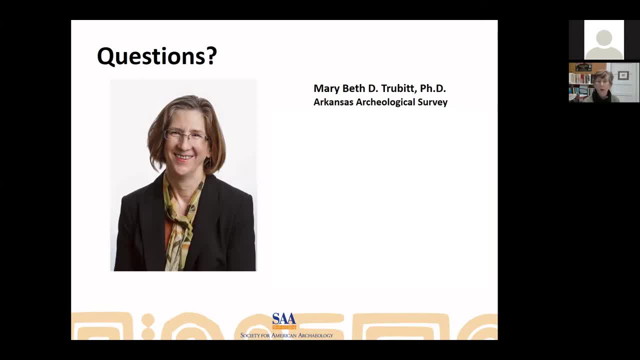 You know, typically you'll include information about where you can access. So what office did you get it from? And that's where it's on file. But you know there's so much accessible And things are accessible, You just have to. 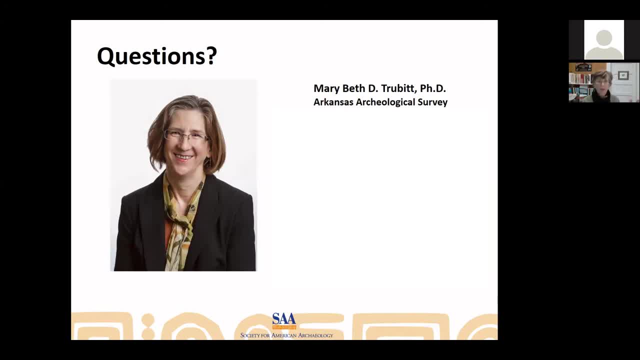 you just have to figure out who in the state has that holds that database. Question: where do I find your handout? That one I'll turn over to Beth. Where do you find the handout? I will be sending up a follow. 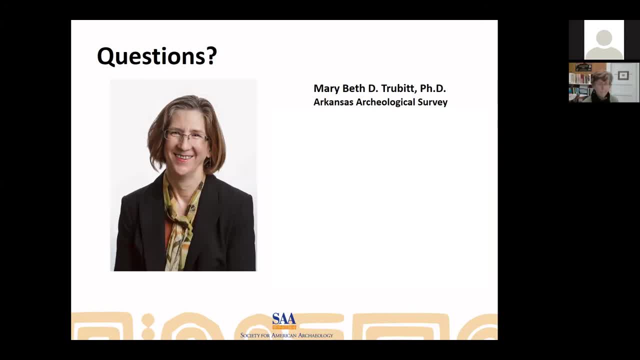 up email to my email address tomorrow to everyone, And it will be attached along with a copy of the slides and where to find the recording of this lecture. Okay, Oh, let me see. Have you identified a target amount of time? Say 250 word. 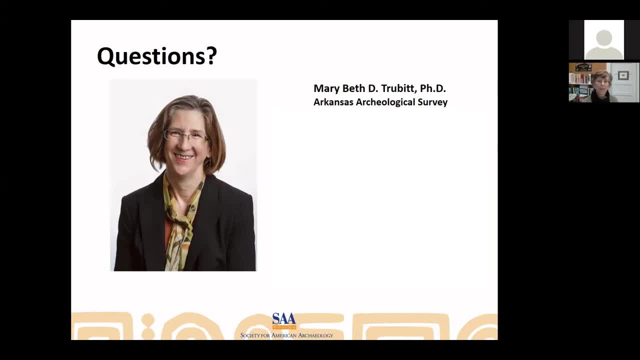 how much time to spend on a standard page. That's tough, You know. you have to be able to spend some time writing. You know I don't tend to worry so much about you know, initially I want to get some words down on the page Because it's a lot. 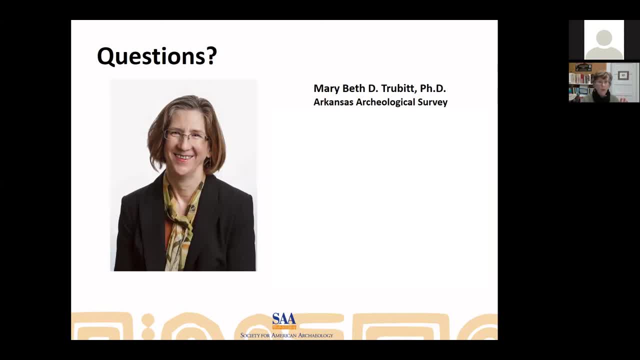 easier to to edit once something's down there than to come up with it in the first place. So get words on the page and then worry about messing around with them. You know I find I don't set a certain amount of time for writing, but I find 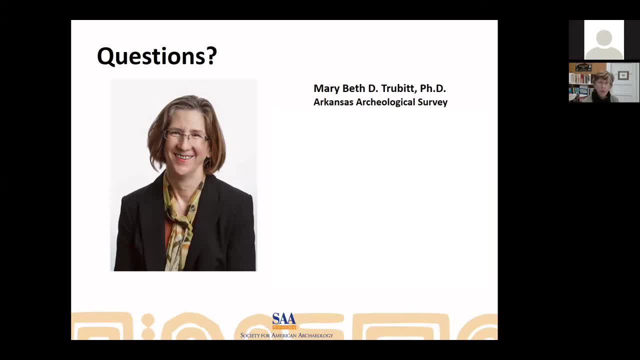 that writing is easier when I'm writing regularly And lately I just got through a three year stint as journal editor And let me tell you: editing, editing other people's writing. now that I have time to write, it's even easier. I'm familiar with 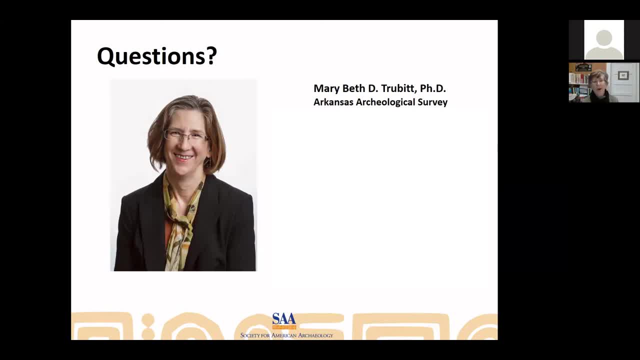 the essay style guide now. So you know I don't tend to try to set deadlines and page expectations for myself. I just try to make it a practice of setting time to write And, you know, allowing myself the time and space. 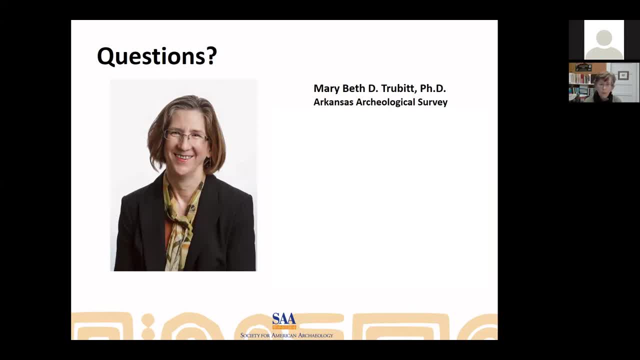 to write Alright. next question: Any suggestions on how to handle historic context concerning minority or repressed groups, For example providing background history as American Indian tribes, when most of the published literature is outdated and somewhat or very racist. You know you have to use 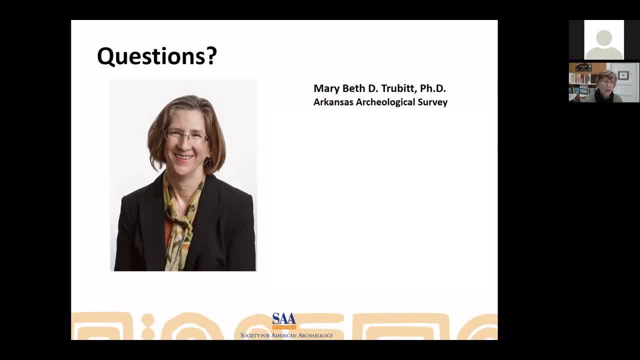 some current material And look at material from different sources. So you know archaeology is a changing field. It is. you know it's dynamic. You can't expect to rely on 40 year old sources and be current, And this is really where 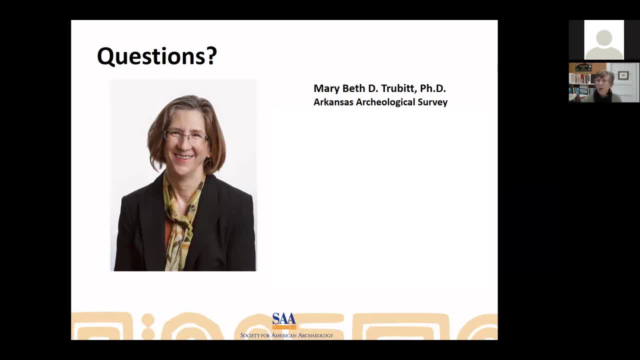 I have a problem with with boilerplate background sections that keep using the same stuff from the 80s and 90s. We've learned a little bit since then. I mean we've come a little bit further, Come on. So, yeah, use. 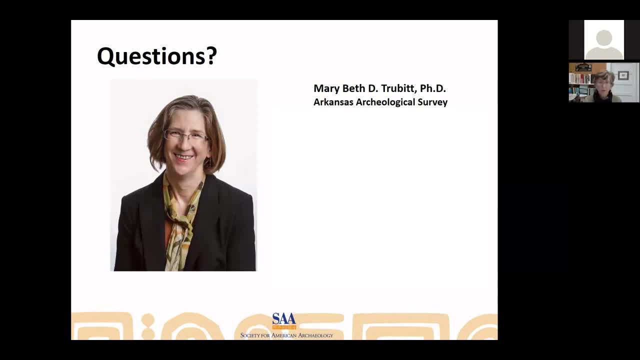 current material and try to get a diversity of resources in there. Keep up with with. keep up with what's going on. Now, you see, the question is really about how much time you schedule for writing. Well, I try to spend at least a couple. 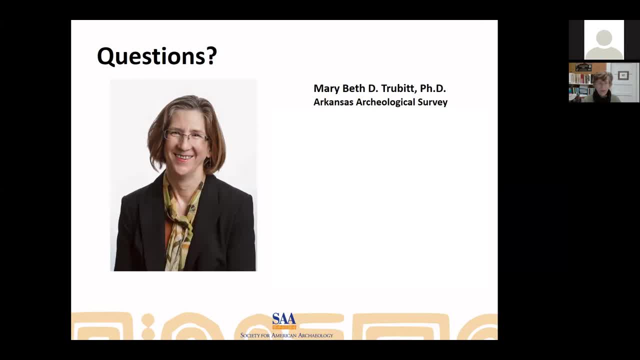 hours. If I'm sitting down to write, I want to spend a couple hours. If I'm serious about scheduling time for writing, I'll come into the office and do it before I check email. I'll make point of checking email midday rather than first thing in the morning. 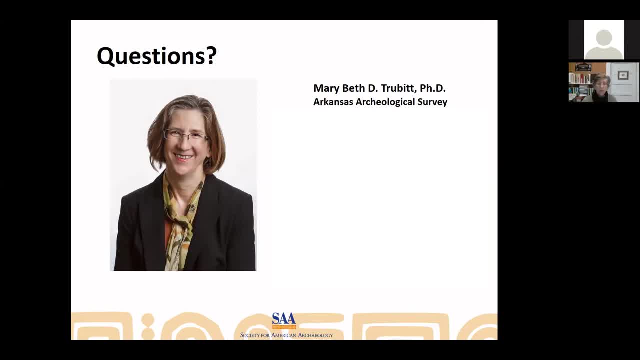 Do you have recommendations or examples for ways to tweak the standard report format for reports concerning collections-based research, specifically with legacy collections, field workers and research that you've conducted decades ago? Well, I've been working. this summer I was working on 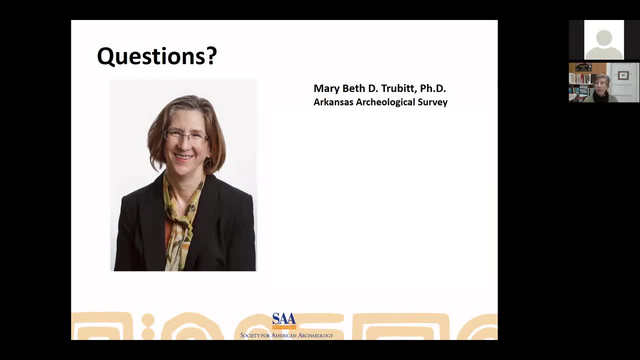 a project that I was actually comparing a site that I had done excavations at with one that a colleague had excavated several decades ago, And for me we actually pulled the material out and did some reanalysis, But for me, structuring it, 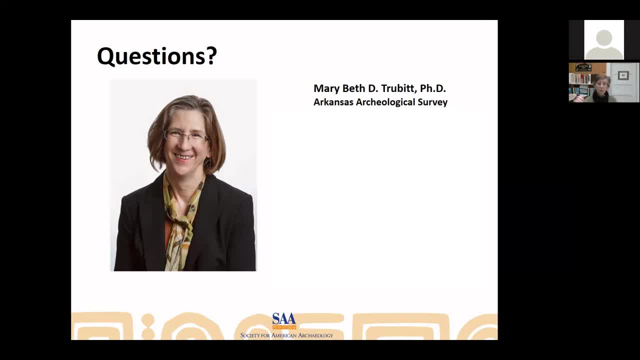 as a comparison between these two sites in neighboring river valleys that were contemporaneous and similar in terms of many aspects made the legacy project more relevant, And so that's how I dealt with that one. Sometimes, the whole can be bigger than the sum of the parts. 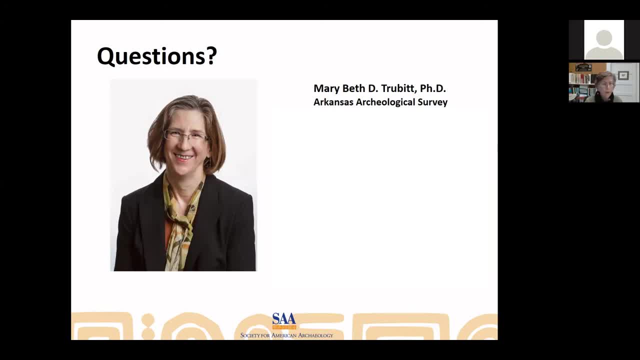 All right, All right. Well, that's all the questions that I see. I think there might be a stray one in the chat. if you've seen that one, Artie, Let me see. Oh, let me see Suggestions about how to disclose. 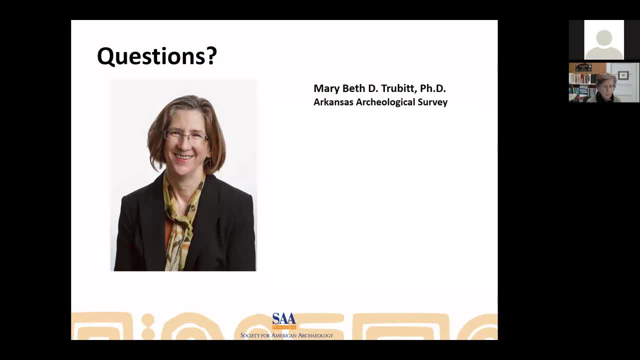 discuss curation and collections, location and accessibility at the various report stages. Decisions about where a collection will ultimately reside are not made before the report is submitted to the reviewers. Um, you know that, yeah, there there are some differences out there, sometimes a CRM. 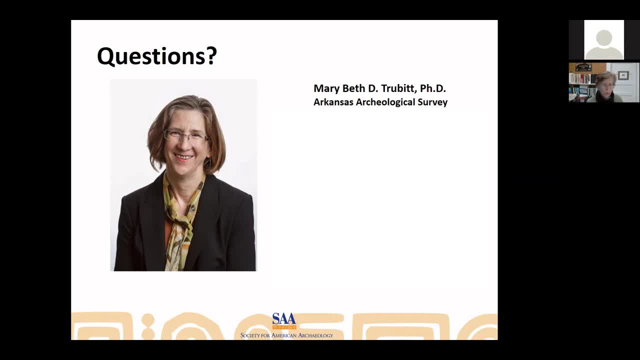 firm may not, may not know where they're going to curate or or something like that. here, you know, here in Arkansas, contractors- yeah, there's a, there's a procedure, there's a procedure and it's included in the in the state standards, and contractors cure, send material to.